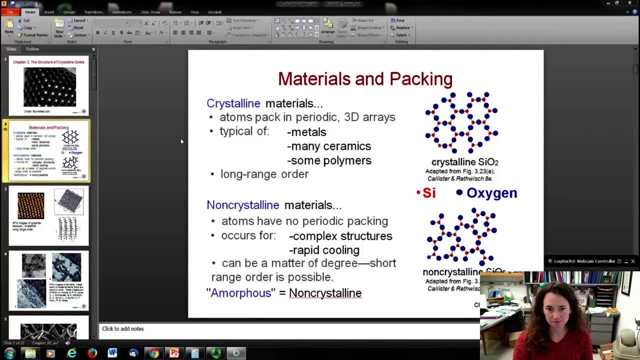 you can get some non-crystalline metals. that way It can also just sort of be a matter of degree. You can have short-range order but not long-range order, And those are often called semi-crystalline materials, A new vocabulary word for you will. 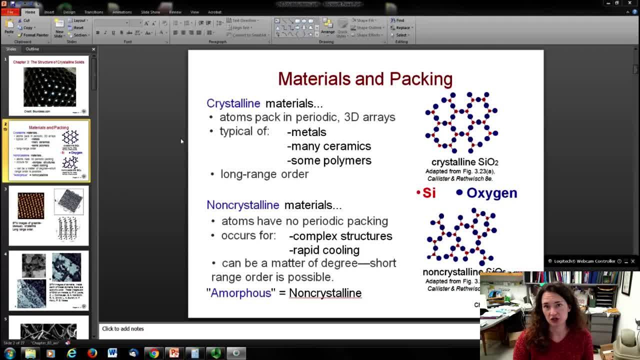 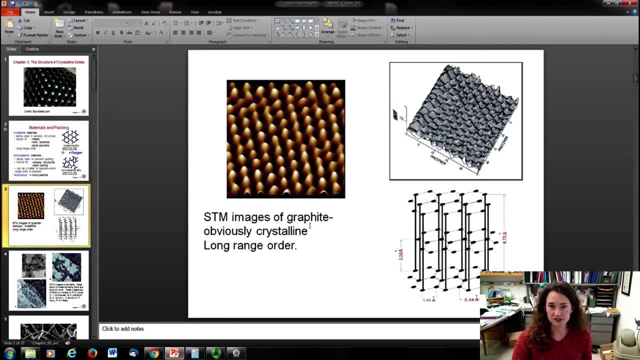 be the term amorphous when we're referring to non-crystalline materials. So here's just a few examples that I have to show you. for crystalline materials. This is a scanning tunneling microscope image of graphite that we took here at Appalachian. 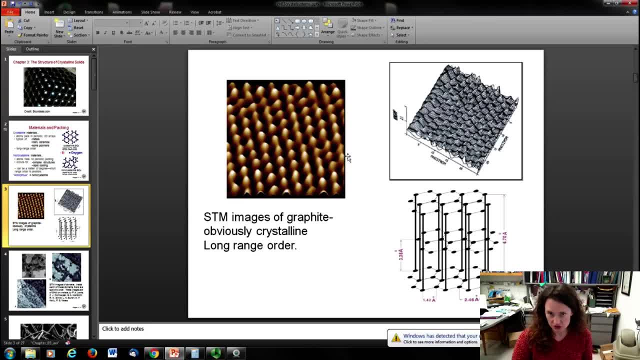 State And you can see here that this is very ordered. So this is obviously a crystalline material with long-range order. If you look at what the structure looks like in sort of a topo plot, then you can see it there. So this is a crystalline material with long-range order. If you look at what the structure looks like in sort of a topo plot, then you can see it there. 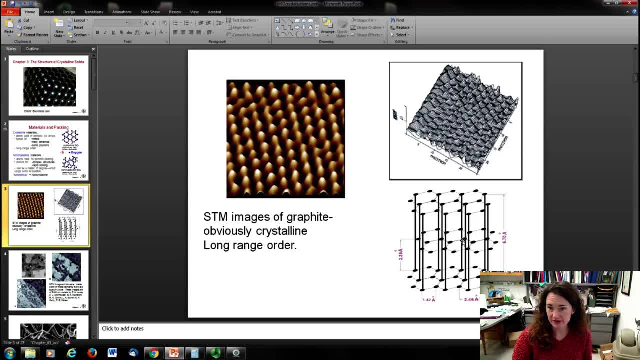 And just borrowing from the web a little bit, this is what the structure of graphite looks like in three dimensions And in STM. obviously you can only see one plane, You can only see one set of atoms, But what happens is in between planes they kind of stack like. 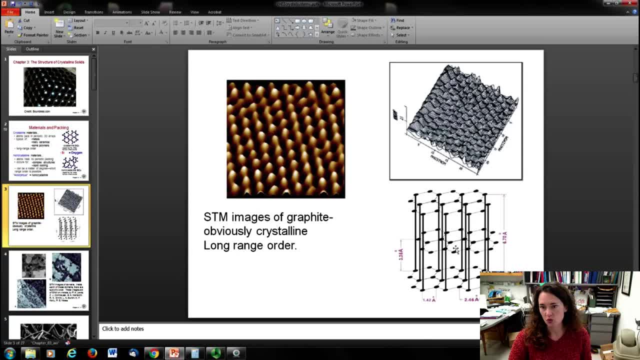 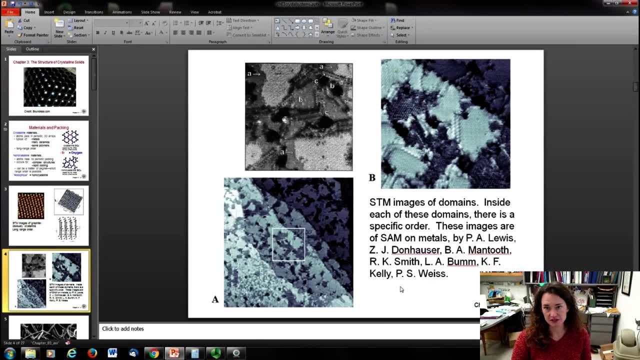 this. So you get a whole bunch of sheets that look like this and they're stacked one on top of the other. Here's some more images. What you can see in lots of crystalline materials is that you'll have a segment called a donor. 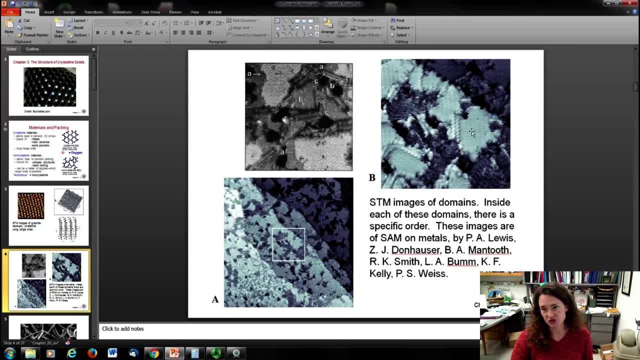 Here's a segment called a domain of the material that has a crystalline structure that looks a certain way, And then right next to that domain will be a domain that's also crystalline, but maybe rotated with respect to its neighbor, And so this is really typical of metals. This 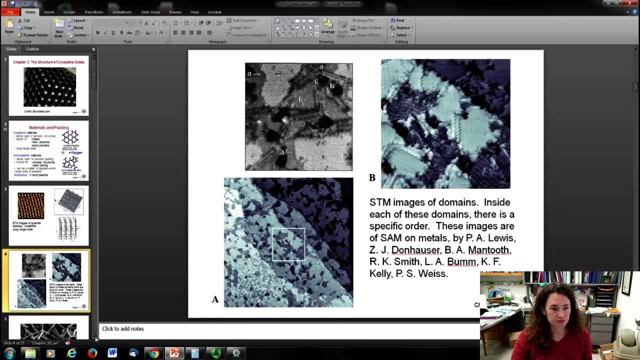 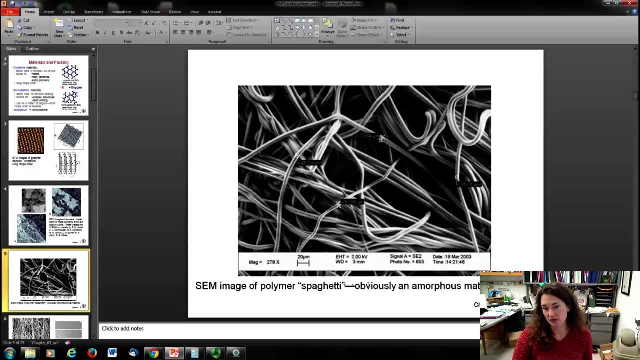 is taken from another publication here This is an example of an amorphous material. This is a scanning electron microscope of polymer spaghetti, So this is obviously amorphous. This is the atomic scale. This is only magnified 278 times, But you can imagine that it must. 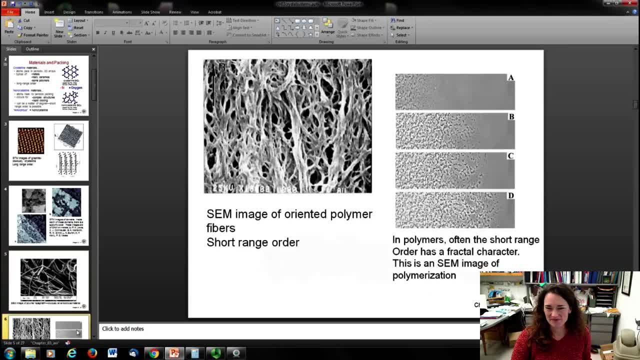 be amorphous just by the way that it looks, And this is a scanning electron microscope image of an oriented polymer fiber. So here you have short range order And you can see that the polymer is growing in a specific direction. You can see here it's oriented vertically on your screen and it's growing. 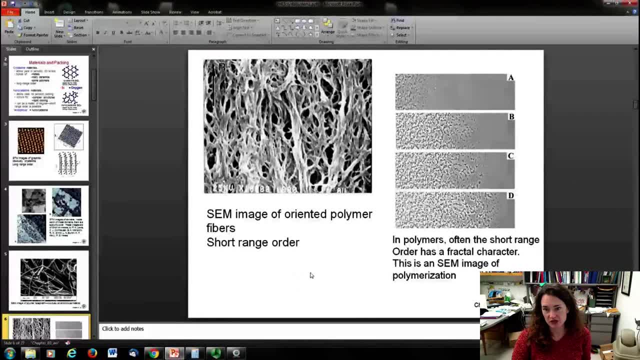 that way And lots of times in polymers the short range order is going to have a fractal character, And this is an SEM time series lapsed image of something undergoing polymerization. You can see it has kind of a fractal structure as it moves out. So that's fun. 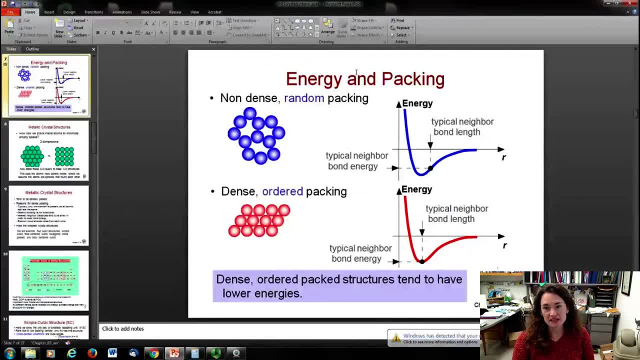 OK, but moving back on for the energies, what happens is in crystal structures for dense, ordered packing, then you're going to have an energy that's going to be minimized. They tend to be very dense, They tend to be very dense, They tend to be very dense. They 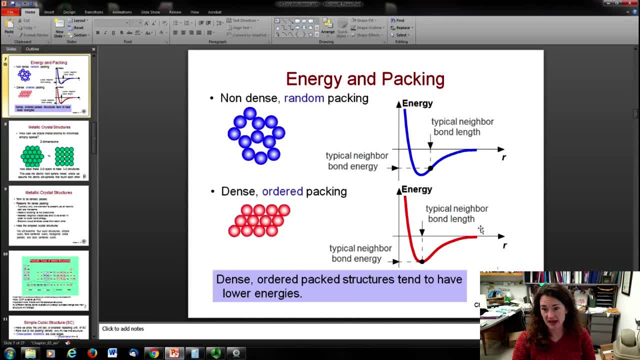 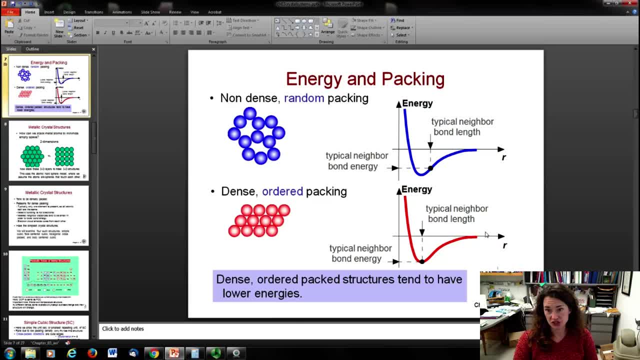 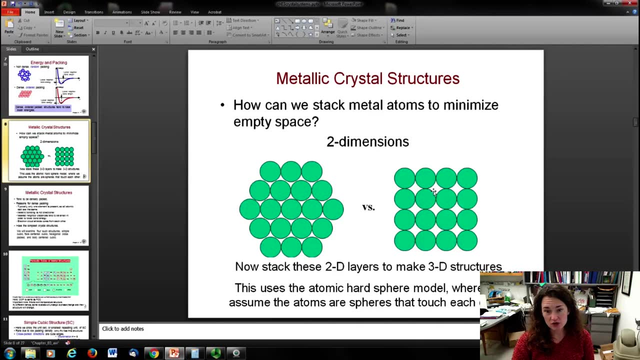 there, at the minimum of this bonding energy curve that you can see. So crystalline structures tend to have lower energies than amorphous structures. Now how do you stack metal atoms to minimize empty space? What we're going to do is we're going to use the hard sphere model, where we assume that 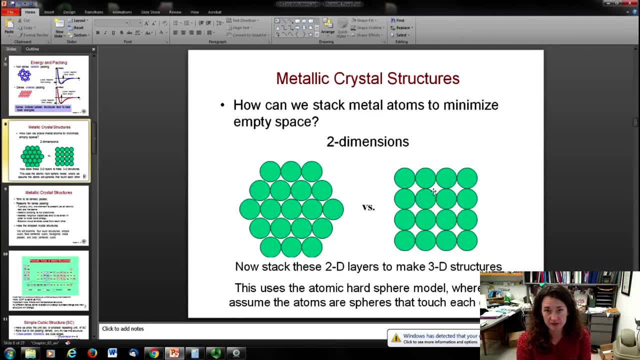 the atoms are basically percolating. But what we did is we're going to do a quick process. We're going to use the hard sphere model, which, you can see, is basically a perfect sphere that has three perfectly fixed spheres that touch each other. Now, of course, this is a model with many flaws, But it does work. 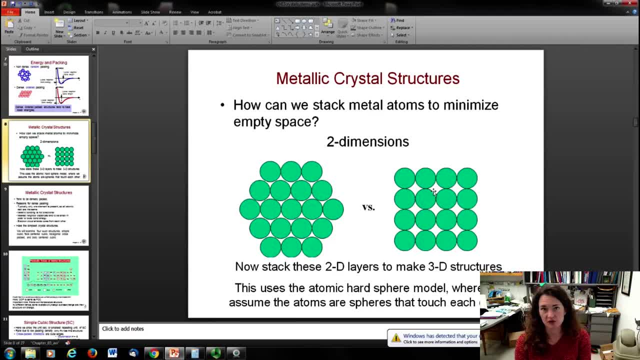 pretty well for describing the metal structures that you'll see in the hexagonal closed pack: face centered cubic. body centered cubic. It explains those structures very well And it's a nice model of metallic bonding where you have the atom and then surrounded by 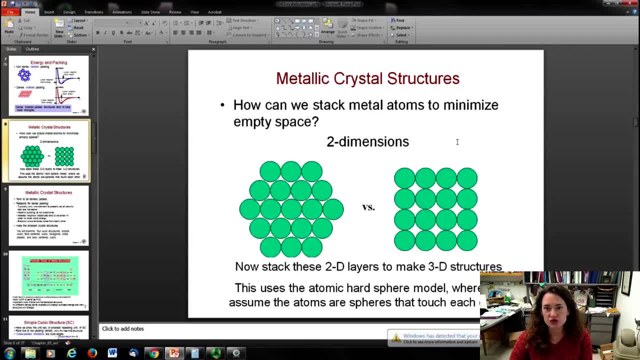 So what you do is you have these two-dimensional structures with these hard spheres, and then what you do is you form a two-dimensional structure and then you add another layer on top of that, another layer on top of that, And so we'll describe in some cases how those layers are packed on top of one another. 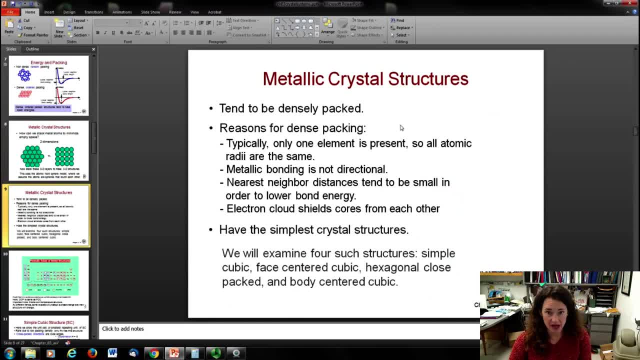 Now metallic crystal structures. they tend to be densely packed. The reasons for this are typically. in the structures that we're going to talk about today, at least there's only one element present, So we'll talk about the structure for copper, for example, or platinum. 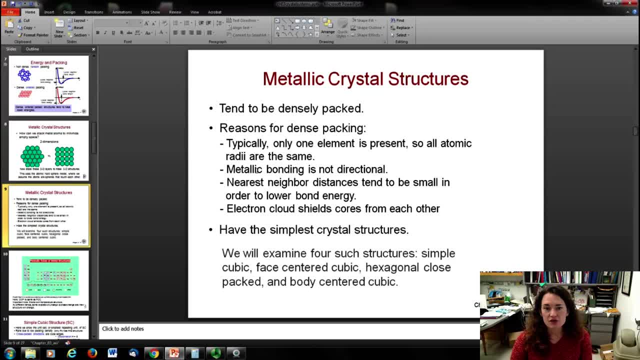 So therefore, all the atomic radii are the same. Also, metallic bonding is not directional. Remember that you have that ion core surrounded by the sea of electrons, and the electron C can go in any direction, which makes the bonding non-directional, unlike covalent bonding. 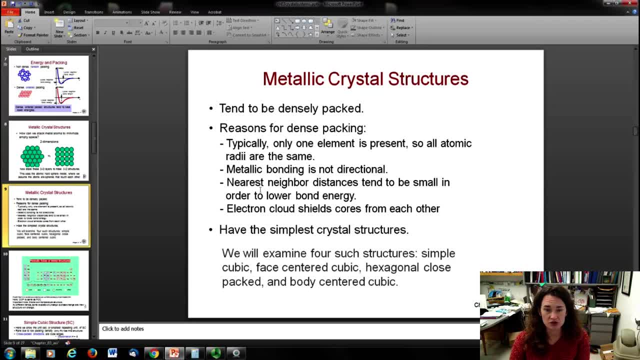 And your nearest neighbor. distances tend to be small. in order to lower that, bond energy in metals, and the electron cloud shields the cores of the ions from each other, And so you have a nice tight, short bond. They also have the simplest crystalline structures, so they're the easiest ones to talk about. 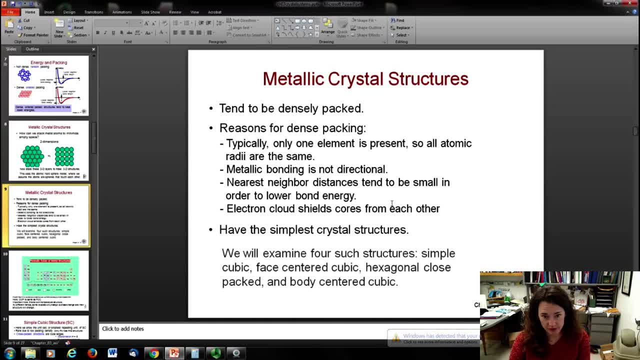 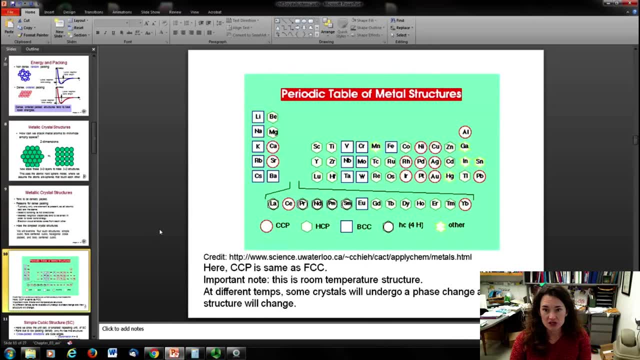 first, The ones that we're going to talk about today are simple cubic, face-centered cubic, hexagonal, close-packed and body-centered cubic structures, And you can see that if you look at atoms that are typically metals, here shown in a periodic table. 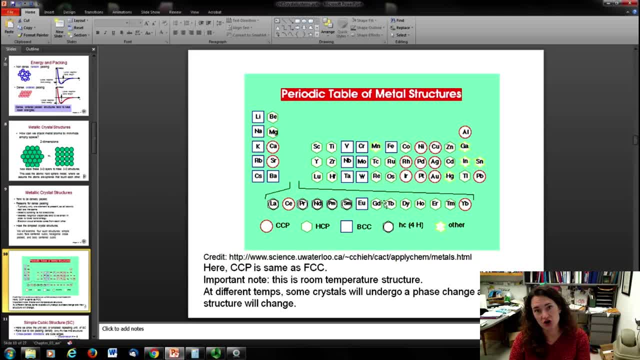 Then you can see what structures are used for these metals. Now here they abbreviate face-centered cubic as CCP instead of FCC, which is what your book does. So you can see that That's in the red, The hexagonal close-packed. the HCP is in the green, body-centered cubic blue and 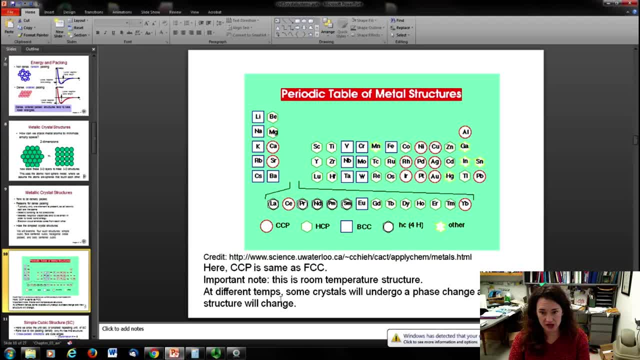 so on and so forth. So you can see them all here in this little periodic table. Now. it's important to realize- and we'll discuss this in later discussions- that the hexagonal close-packed, the HCP, is in the green, body-centered, cubic, blue, and so on. 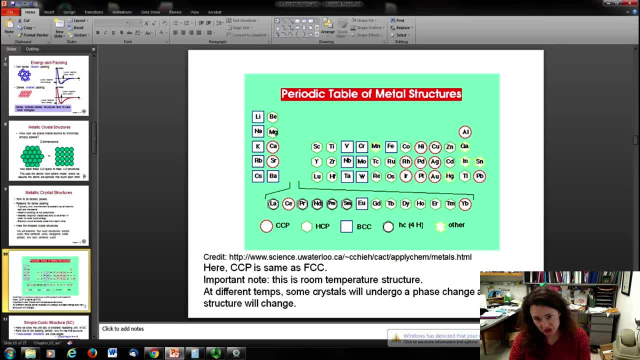 and so forth. So you can see that in later chapters that at different temperatures, some crystals are going to undergo a phase change Now, unlike a typical phase change where you're going from a solid to a liquid, which is kind of what we discussed in introductory physics courses 1150,, 1151, crystalline structures. 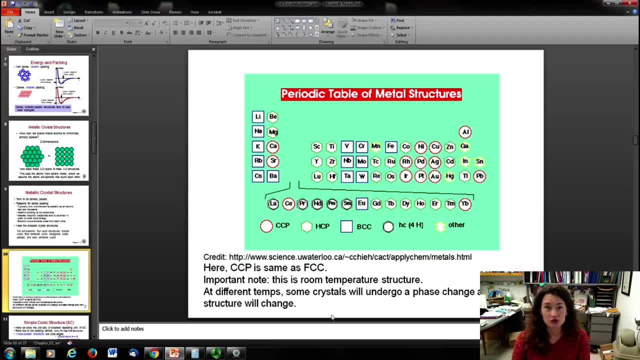 can undergo a phase change from one type of crystalline structure to another type of crystalline structure. For example, iron will go through phase changes and go through from an alpha to a gamma phase, and that changes the structure. So you can see that. 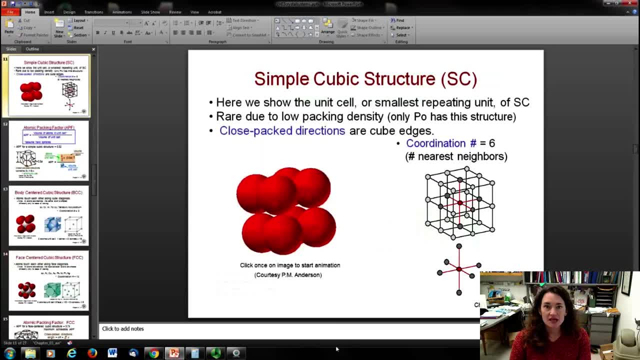 So that's kind of interesting. So the first one that we're going to discuss is the simple cubic structure. Sometimes it's abbreviated SC. It's the easiest to talk about because it's the simplest structure, so we always do it first. However, I do want to note this is a pretty rare crystalline structure, and the reason 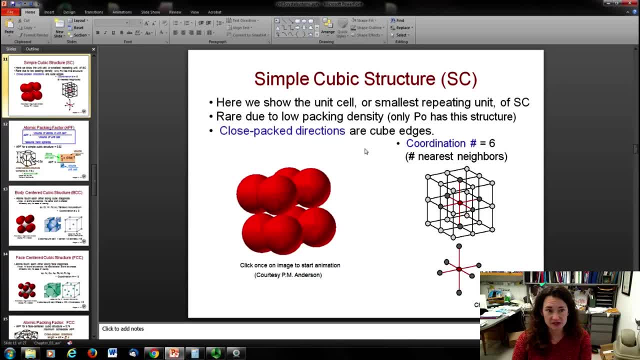 is that it has a very low packing density. So out of all the ones in the periodic table, only polonium has this structure. So the close-packed directions are the cube edges And those are the ones with the highest packing density. Inside the cube it's kind of not taking up much space with solids there. 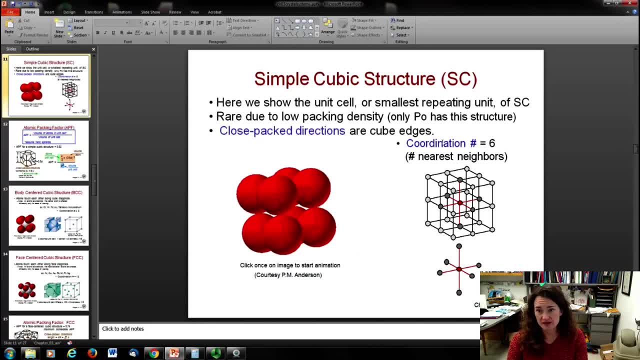 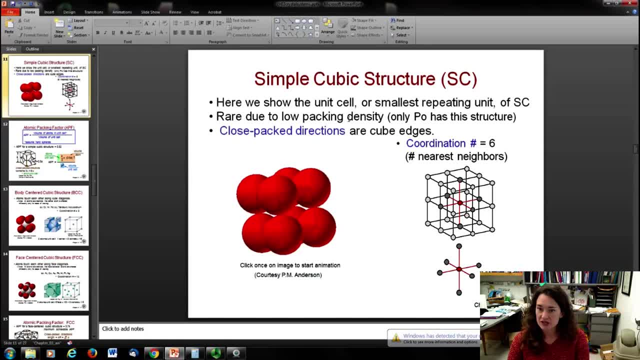 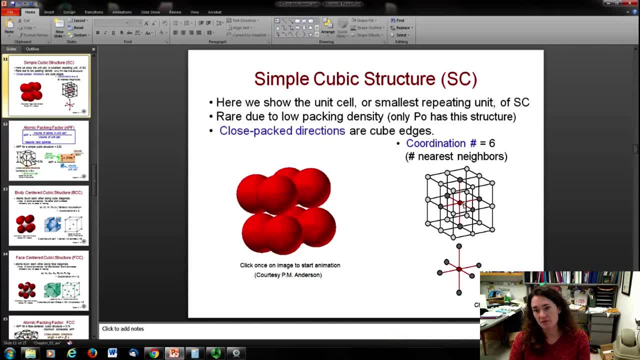 And you can see that each corner of the cube is going to touch six other neighbors in the shortest possible distance. Okay, So, for example, if you look at the one that I'm sort of highlighting and pointing to here and now extrapolate what that would look like in a larger three-dimensional array, 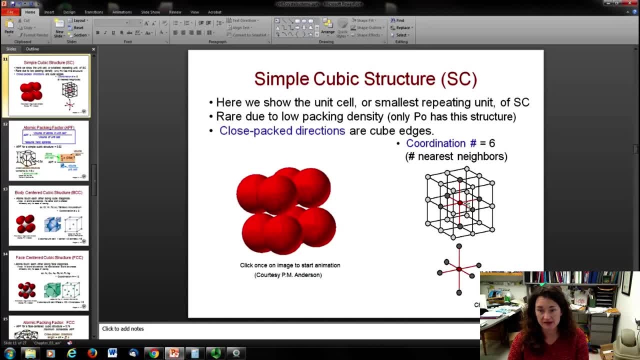 it would touch six other neighbors in that way. So the coordination number is six. okay, now, here we're going to show the unit cell, and the unit cell is the smallest, simplest structure that shows all the bonds. okay, so here the unit cell is a little cube, of course, and the atoms are pictured at each one of the cube. 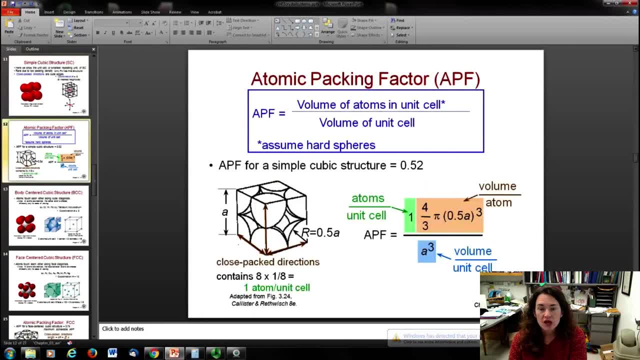 corners. another thing that we want to define and as often talked about for crystalline structures, is the atomic packing factor, and it's abbreviated in your text as APF. the APF, the atomic packing factor, is the volume of the atoms in the unit cell divided by the volume of the unit cell. so basically, 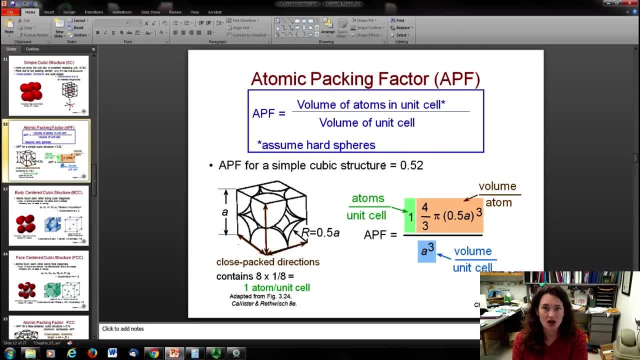 it's just a fraction that shows how much space is occupied inside the cell. now APF for a simple cubic structure is 0.52. so let me go through as an example how you would do that calculation for an atomic packing factor. first you would multiply. 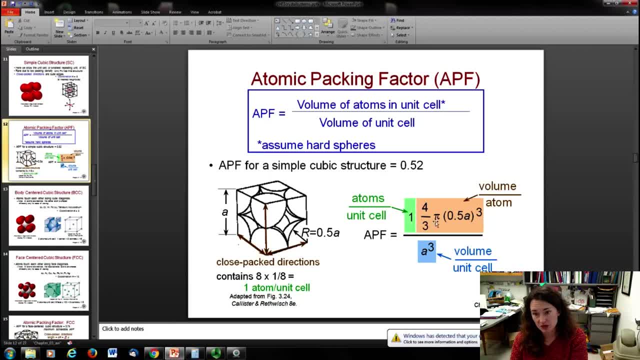 the number of atoms in that unit cell by the volume of the atoms in that unit cell, and then you would multiply, times the volume that each atom has and then you would divide by the volume of the total cell. now, oftentimes in your book they talk about the length of the unit cell. now, this is a cube, so in each direction. 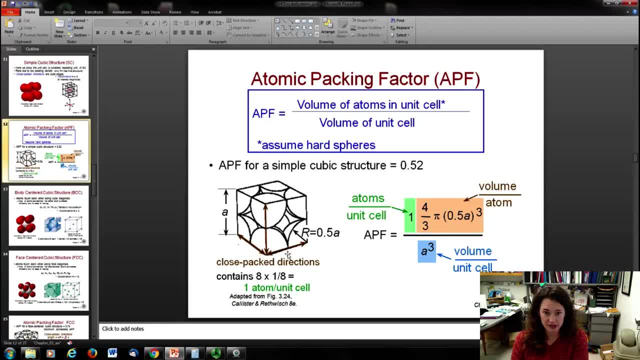 along the edge. it's all. a a is the length of the cube here. okay, now if you look at what it looks like within the cell, then each corner of that cube is going to slice through one of the atoms. okay, so the cube is made by connecting center to center of all the atoms in the 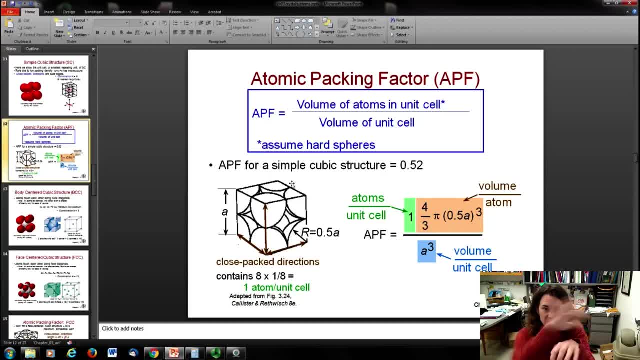 cube and when you do that you're going to cut off part of the items. part of the atoms are going to stick out. so at each corner here see, you have eight corners to the cube and at each corner you've got 1, 8th of an atom. okay, 1 8th of an. 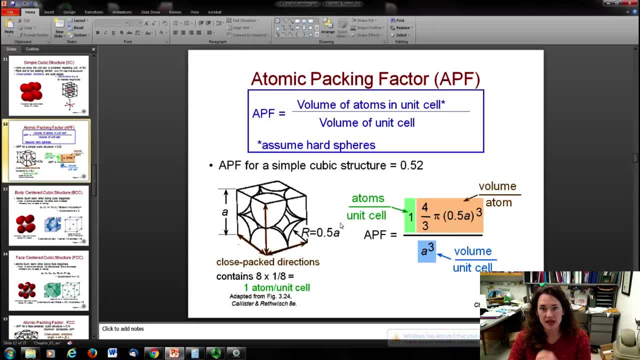 atom. so the number of atoms per unit cell is the 8 corners times the 1, 8th, which gives you, for a simple cubic structure, one total atom per unit cell. now, the volume of the cell is the volume of an atom if you assume a hard sphere. 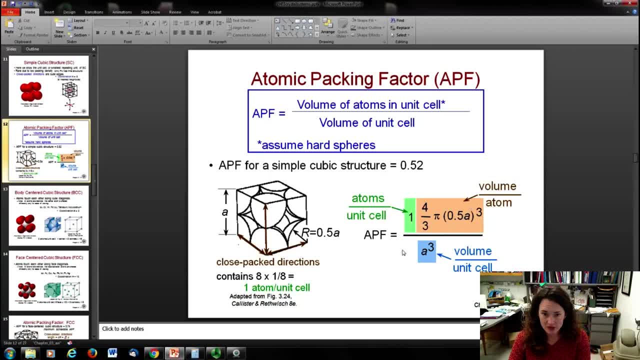 model, the volume of a sphere is 4 3rds pi r cubed, but the radius of each atom is actually going to be equal to half of the length of the unit cell. you can see, here you've got two atoms touching at the bottom corners of the cube, and a is. 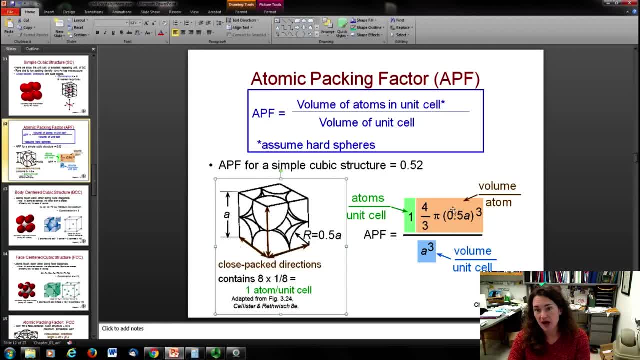 equal to 2r there. okay, so 4 3rds pi times the radius cubed would be half of a cubed and you would put that on top and now, because it is a cube, you're going to be able to see that the volume of the unit cell is just going to be length. 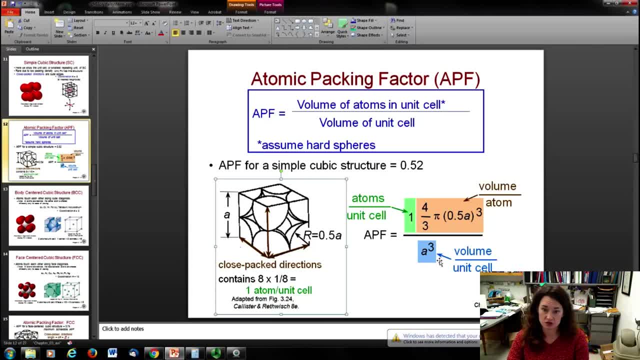 times width, times height, all those are the same. they're equal to a. so it's a cubed. now if you multiply all this stuff, divide numerator by denominator, then the a's cancel out and you end up with 0.52 for the atomic packing factor for a. 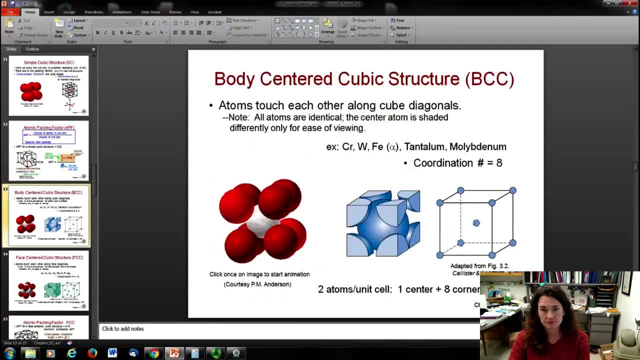 simple cubic structure. okay, the next one up is the body centered cubic structure. this is all often abbreviated BCC. the thing is here, the atoms at the corners of the cube are no longer touching each other, unlike in the simple cubic structure, and that's because you've got this atom right here in sort. 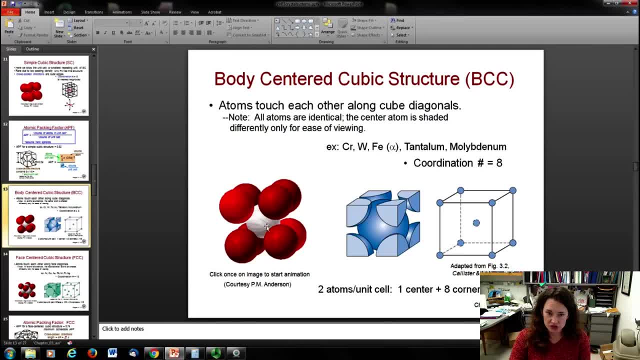 of the middle of the cube. so all the atoms on the corners are touching the one that's on the inside. there examples of metals that have this structure: chromium, tungsten, alpha phase of iron, tantalum, molybdenum, so on and so forth. the coordination number here, the number of nearest neighbors for each atom, is: 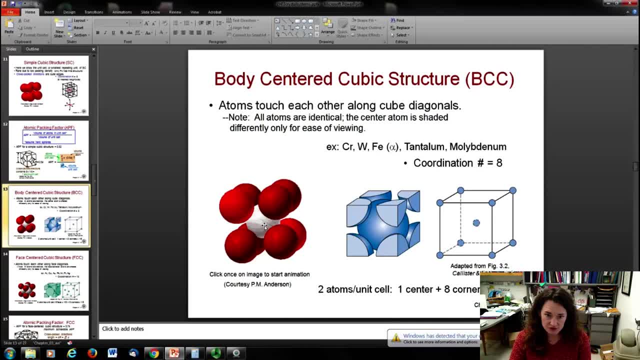 eight. so you can look at that. the one in the center of the cube is touching all these other atoms on the corners, and of course there's eight corners to a cube, so the one in the center is touching eight. okay, so the coordination number or the number of nearest neighbors for each atom is: 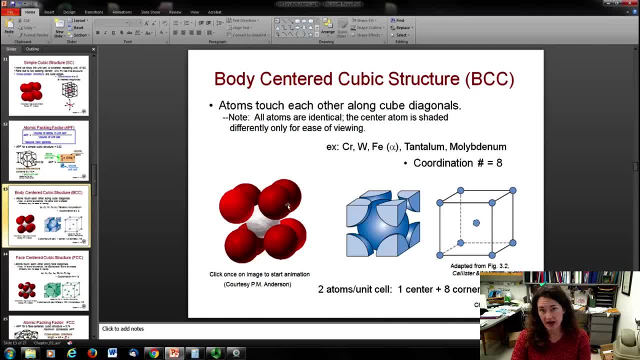 eight, because of course, you can consider any one particular atom to be at the center of another cube. okay, if that makes sense. now this one is going to have two atoms per unit cell. all right, you've got the one in the center, of course, and then you add that on to the corners of the cube. 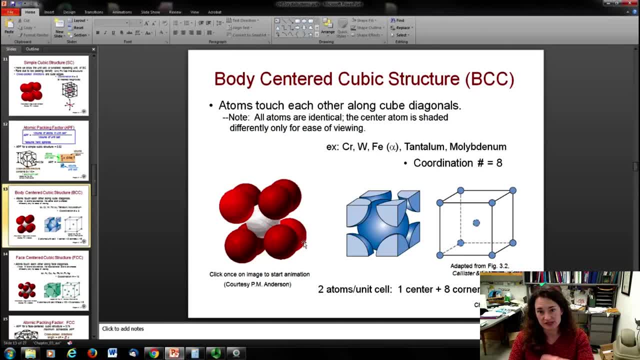 okay, which is of course eight atoms at the corners of the cube, but they're going to be sliced off, so that's times one, eighth, so the two in the center, the one in the center plus the one, the one atom that comes from all the corners, and 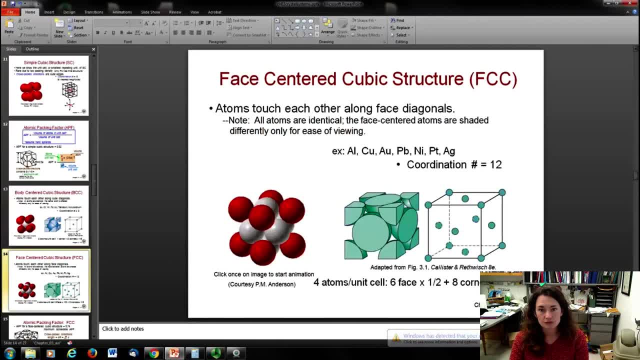 that gives you two atoms per cell. okay, the face centered cubic structure. in this one what you have is, of course, the atoms of the corners of the cube. but then you have an atom that's sitting at the center of each of the corners of the cube, face of your cube. Now, in this one there's no atom in the very center, just the ones along the. 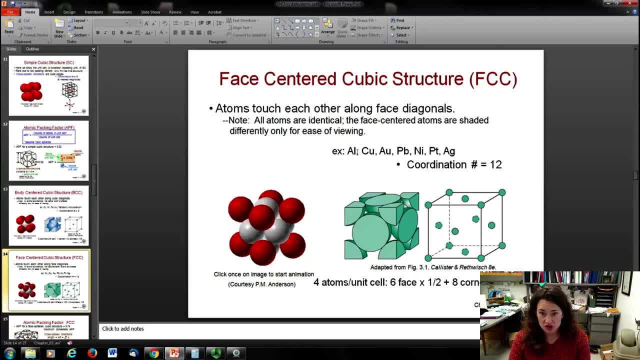 faces. all right, Some examples of this structure: aluminum, copper, gold, lead, nickel, platinum, silver. This one has a much higher coordination number, So, to explain this, the coordination number is 12.. So if you look at this atom here on the center of this right-hand face, 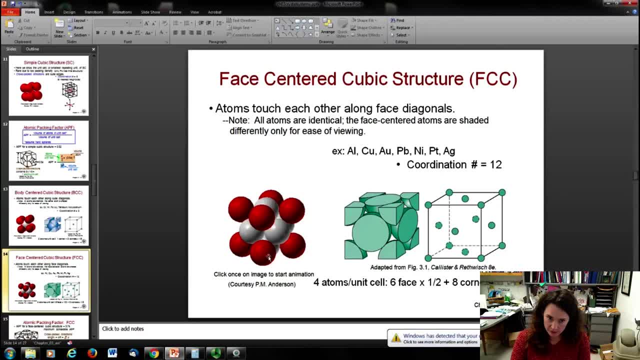 it's touching the four at the cube, the corners of this side of the cube. It's also touching each one of these guys. that's hitting the face of the front and the back and the top and the bottom faces. It's also touching those. And then, of course, if you kind of move it out and imagine, 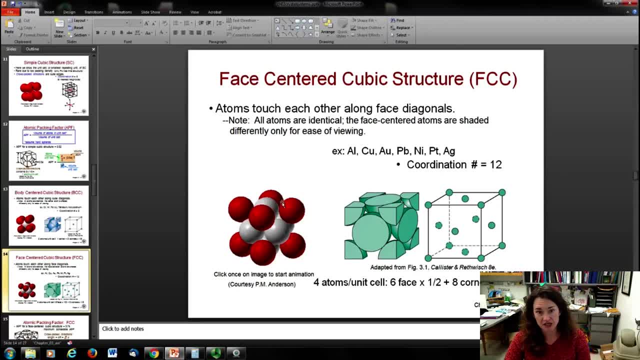 that you have an array of these little structures. it would be touching the four gray atoms from the neighboring cube. okay, And 4 plus 4 plus 4 is 12.. So the coordination number is 12.. The FCC structure also has a higher number of atoms per unit cell. okay, Each one of. 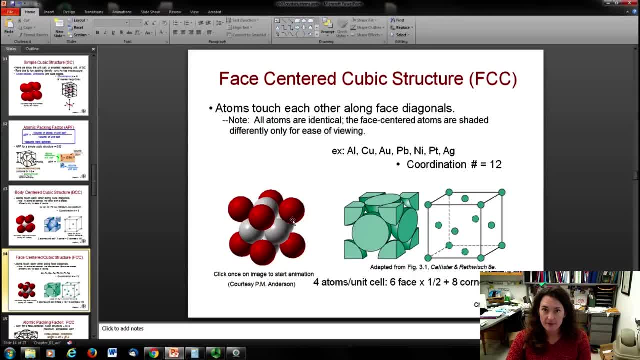 these atoms that sits on the face, all right, is going to get sliced in half, And there's six faces, So 6 times a half gives you 3.. And then plus the atoms of course at the corners, times 1, eighth. So that's 8 corners times 1. eighth gives you 1.. So that gives. 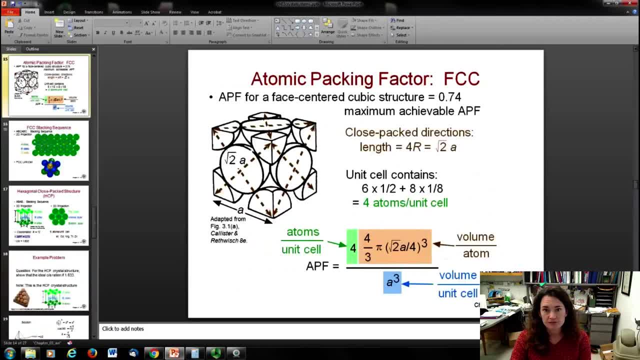 you 4 atoms per unit cell. Let's go ahead and calculate the atomic structure, The atomic packing factor for an FCC. The atomic packing factor of the APF is 0.74.. I emphasize this because it's the maximum achievable atomic packing factor that you. 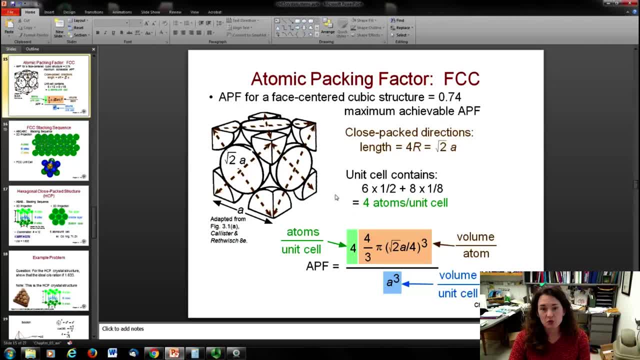 can get All right. So, remembering that you want to multiply, for an atomic packing factor, the number of atoms per unit cell times the volume of an atom and then divide by the volume of the cell. all right, We already talked about the number of atoms per cell, That's 4, okay, And the volume of 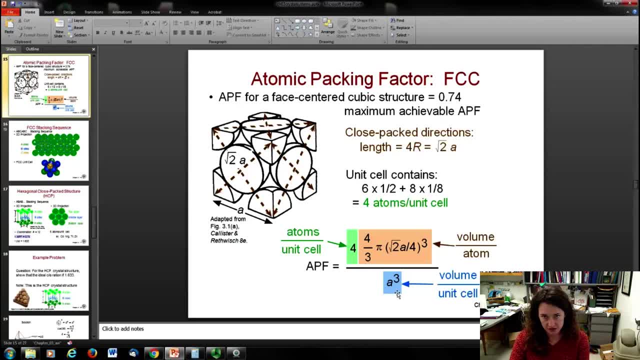 your unit cell is a cubed, just like an atom. So the number of atoms per unit cell is a cube, just like an atom. So the number of atoms per unit cell is a cube, just like an atom. And then the volume for an atom would be 4 thirds pi? r cubed. Now, in order to figure: 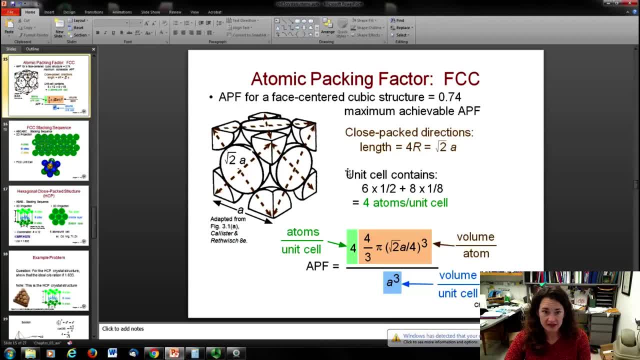 out what r is in relationship to a, then we can look kind of along this face right here. Okay, So you can see that along this face you've got one radius from the corner to the atom on the center of the face And then the atom on the center of the face you've got 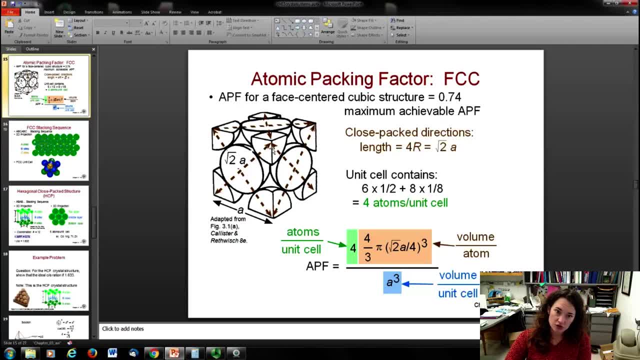 two radii right, And then another corner gives you another radius, So that's 4r: 4 radii across the diagonal of that cube And then the diagonal, of course, of a square. here you have a square where you 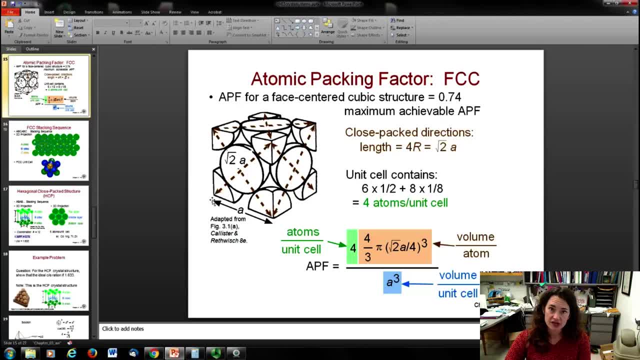 have a side a and a side a right here And if you go across the diagonal that's equal to the square root of 2 times the length of the side. So that's root 2a across that diagonal. So here you have: 4r is equal to root 2a and you can solve for r in terms of a and plug that in And you. 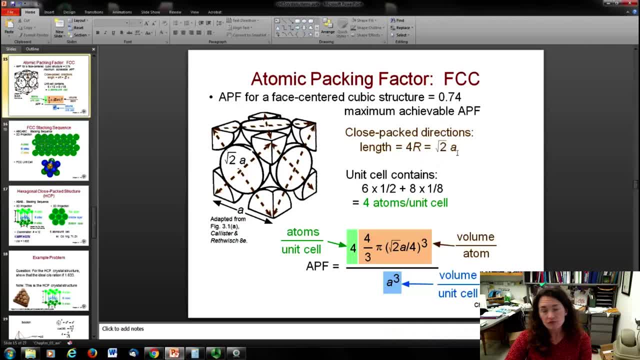 would get r is equal to root 2 over 4 times a. So now if I plug that into my formula for the volume of an atom, 4 thirds pi over cubed, then I have 4 times 4 thirds pi, times root 2a over 4. 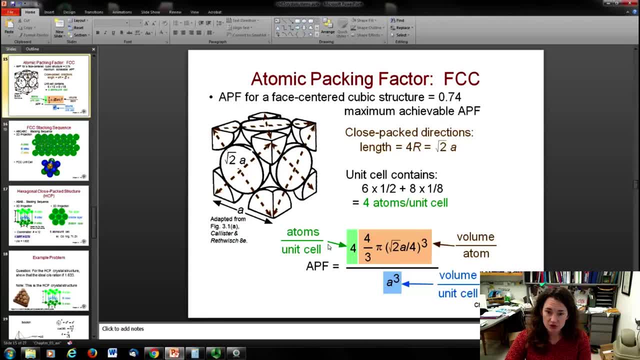 cubed and then divided by a cubed, And then when you multiply all this stuff out, the a's cancel and you end up with 0.74 for that ratio for your atomic packing factor. I'd like to add that sometimes, especially if it's been a while since you thought about geometry, for 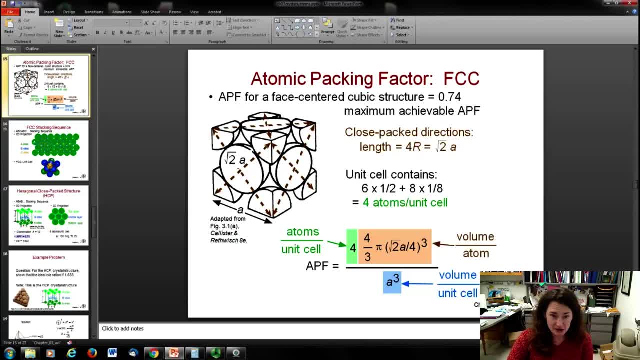 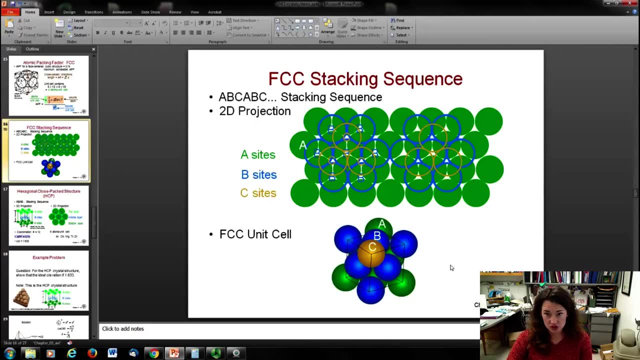 this stuff. you should probably pause me and go and stare at it real hard until you make sure that you can understand what I'm saying. That's the beauty, though, of an online lecture: You can always pause the talker. Let's talk about the stacking sequence for an FCC structure, So remember, 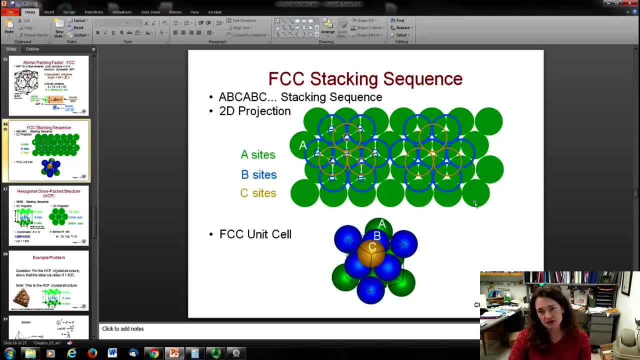 we talked about adding things and layers, And so if you think of the green layer here as the one on the bottom, we'll call that a, And then the b sites. that's the next layer that you would add on That's shown here, And then the b sites. that's the next layer that you would add on. 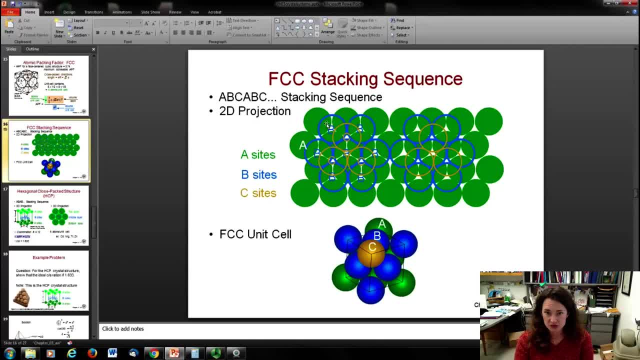 That's shown here, And then the b sites. that's the next layer that you would add on. That's shown here in blue. And what happens is you just put the balls into the minimum point right here in between, forming a little pyramid between the bottom and then the next layer up, And you 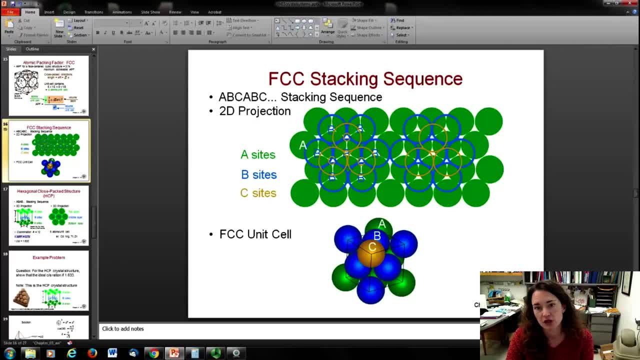 continue to do that, so that all the atoms from b sit in the little low points from the atoms from a, And then you do the exact same thing again for c. okay, For the next layer. you put the orange layer here into the minimum points on b. So what would happen is this is the structure that you 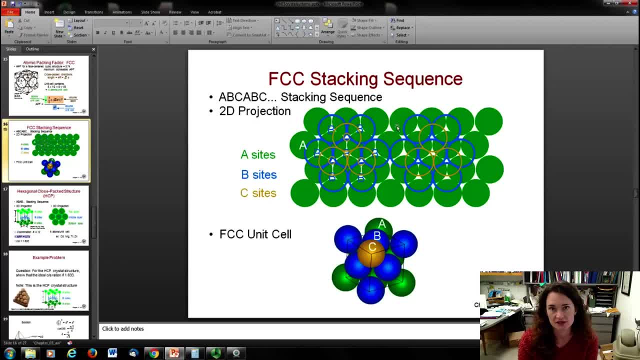 would get, for example, if you threw a whole bunch of ping pong balls into a box and gave it a shake until it settled out, all right, And then you have your FCC unit cell, And then what would happen is you would have to turn that on its side in order to see the cartoon that I showed you on the 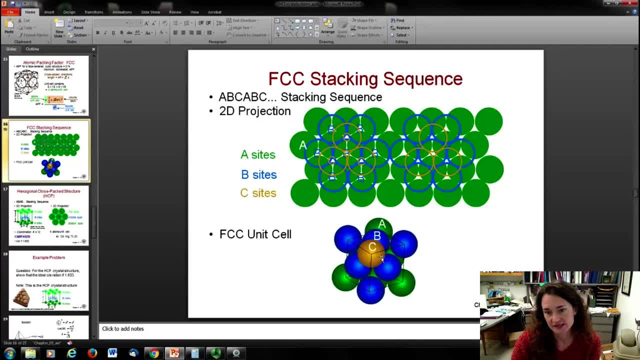 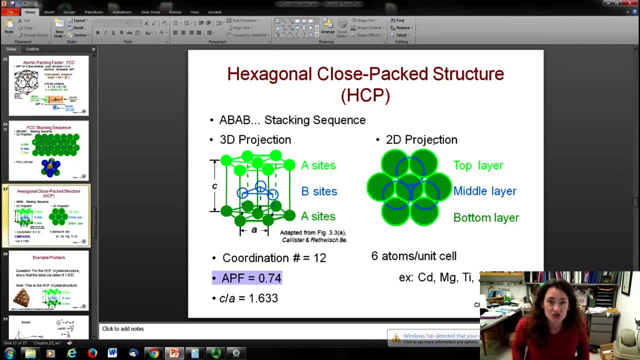 previous page. It's pictured here And there's your a, b and c atoms like so, all right. The hexagonal close-packed or HCP structure is the next one on our list. This one has an, a, b, a, b stacking sequence. all right, The structure of this one is slightly 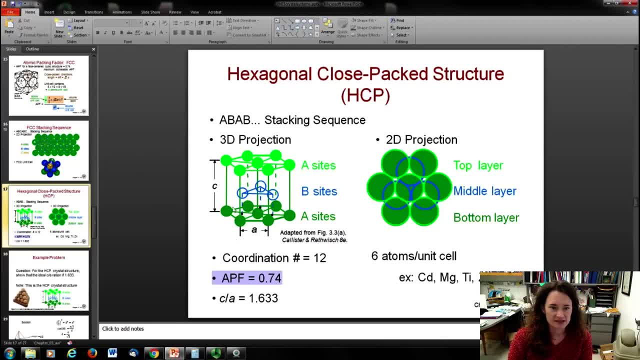 different. Here you see a very hexagonal looking thing. You have a hexagon here and then you have an atom at the center of the hexagon. All of the atoms nearest neighbor distances are a, as shown here. And then in your next site you've got atoms sitting in the minimum. 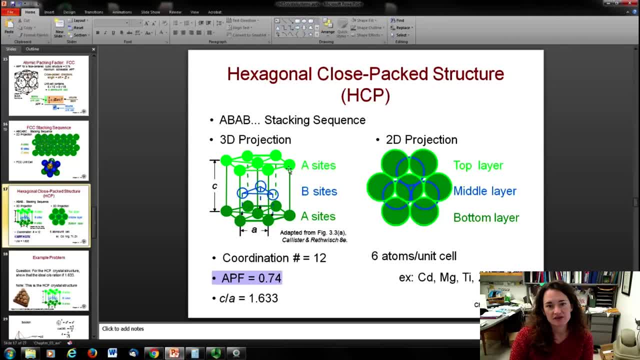 points in between your hexagon right here And then you have another structure right here that looks the same as the bottom. So oftentimes they show the HCP structure as sort of an upright solid, that's sort of a hexagonal prism that pulls up, And so what they talk about is the c over a ratio. 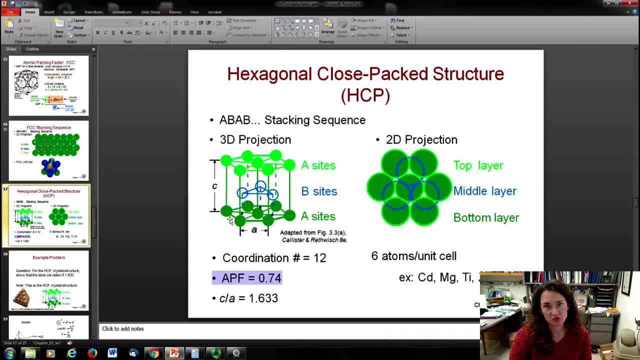 I'll derive it for you in a second. But the c over a ratio would be the height of that prism, c divided by the nearest neighbor distance between the atoms, which is the length of one side of the hexagon, which is a here. all right, 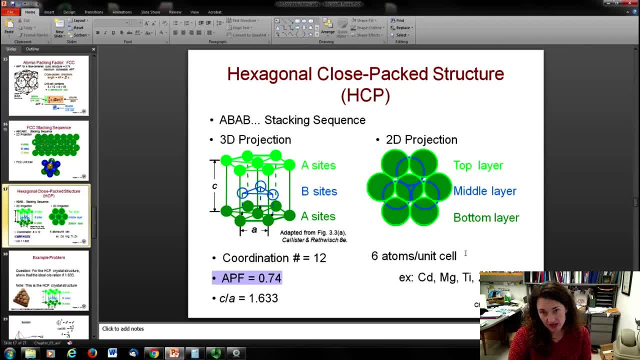 Now this one has six atoms per unit cell. It's probably easiest to really stare at it to see why. okay, You've got your three on the inside here, and then you have the ones that get sliced off from the top and the bottom layers, all right, And the coordination number is 12, just like in. 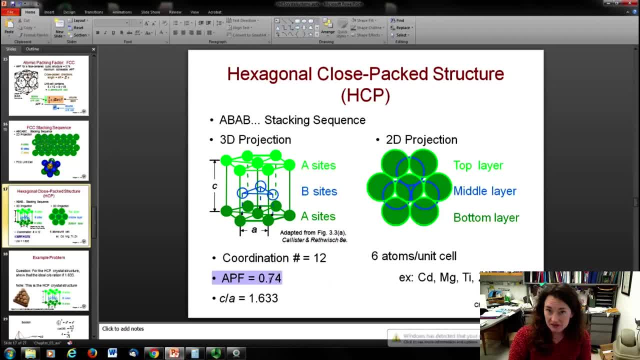 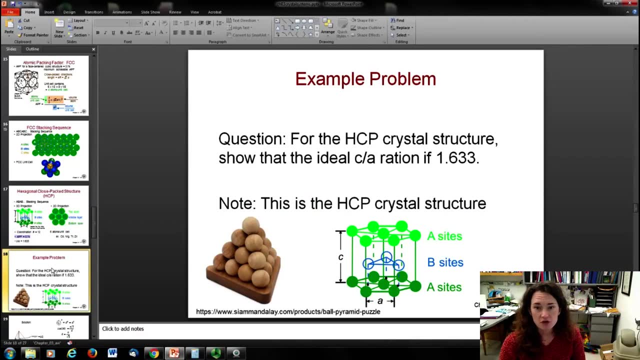 an FCC structure. The atomic packing factor, also like an FCC structure, is the maximum achievable, which is 0.74.. All right, let me do an example problem concerning the HCP crystal structure. So the question for this example problem is for the HCP crystal structure. show that that ideal c over a ratio is 1.6333, okay. 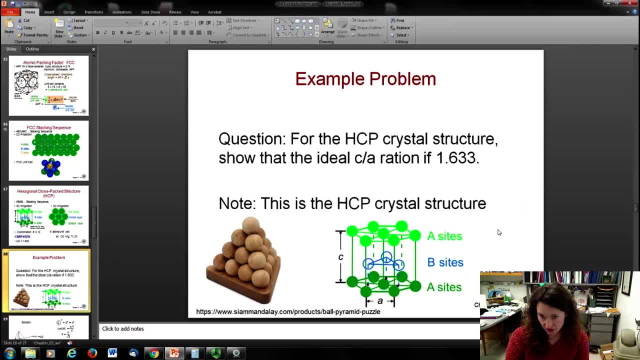 So note, this is the HCP crystal structure. okay, Here you have your hexagon, and then your little triangle in the middle and your hexagon on top. Now, if you think about it, this little b site is the base, and then the middle atom here on the top is forming the pyramid. So that's the structure. 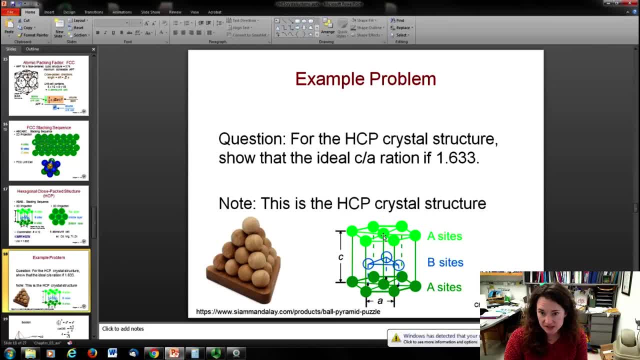 I'm going to go back to This middle atom in green in the top sits in the minimum point of this little triangle right here. So it's kind of, if you want to picture it this way, like forming a little pyramid made out of balls and you're just looking at the top four atoms in that pyramid. okay, 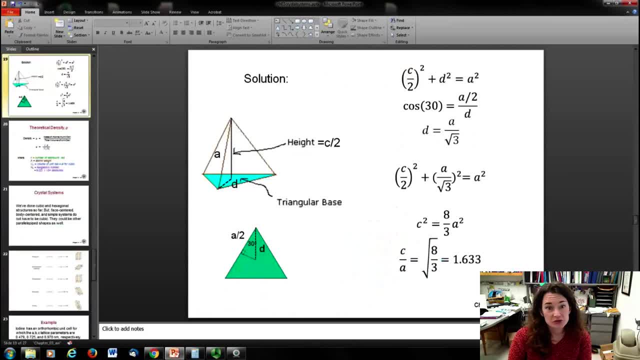 Symbolized here. So I'm going to do a little bit of geometry to solve all this. Here's my little triangular pyramid that I was talking about, which is the very tip top of the ball pyramid shown on the previous page, At each one of the corners of this little prism here I've got. 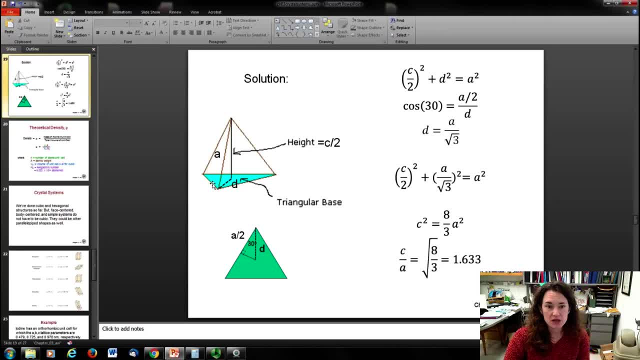 or pyramid. here I've got an atom, okay, Now this is an equilateral triangle here on the bottom of the atom or on the bottom of the pyramid, And then the top atom sits in the minimum of that sort of valley right there which is going to be at the very dead center of that equilateral. 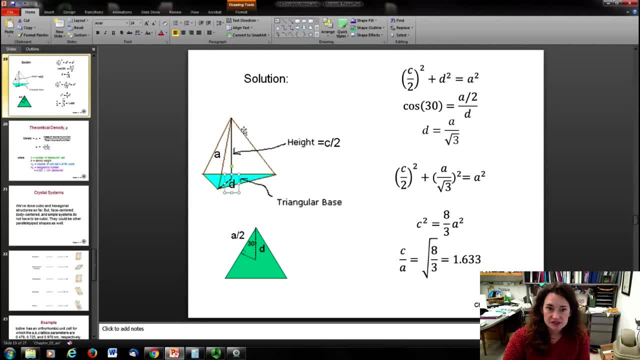 triangle. okay, Now the nearest neighbor distance between any two atoms in an HCP structure is A. okay, It's also the sides of one of those hexagons, So A here is going to be the distance in between the very top of that pyramid and then along the diagonal of the pyramid to the atom here on this side. okay, So 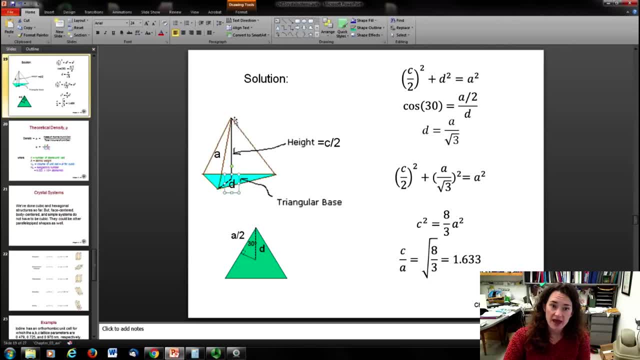 that's A. Now if I drop a line, a plumb line, basically from the top of the pyramid to the bottom right there, then that gives me okay. So that's the height of your hexagonal prism over two, because of course it has that. 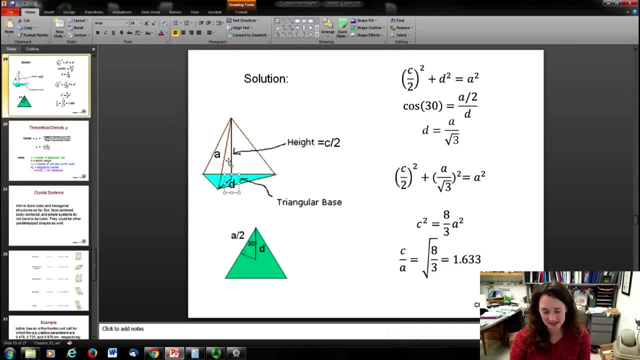 A, B, A, stacking, okay, And so you're only going from A to B. You're not going A, B, A, okay, So that's half, So that's C over two, all right, And now D here would be the distance from this. 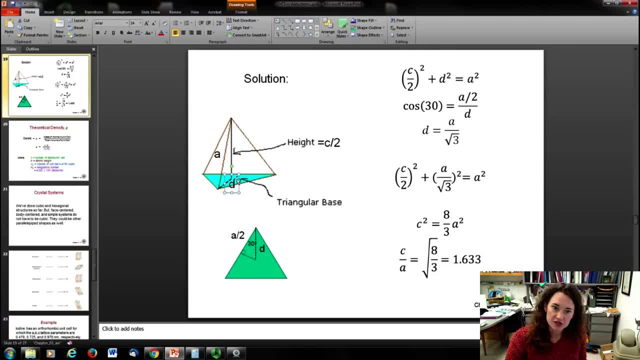 corner of your pyramid right here to the midpoint of the base. okay, So that's my prism pyramid. now, if I look at this triangle right here which is formed from the top of the pyramid to this corner and then along D here to the plumb line, 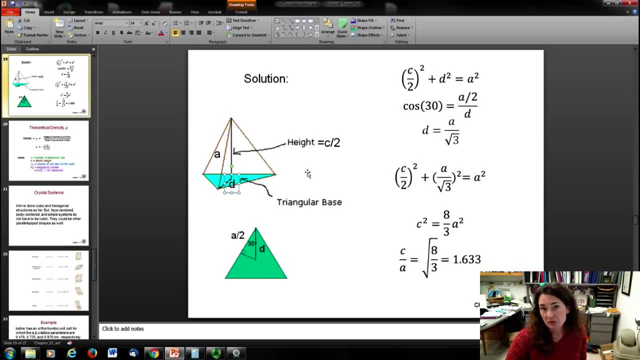 C over 2. okay, so if I look at that triangle, then I can apply the Pythagorean theorem to that triangle and what I've got is that the square of the sides of this right triangle will then sum to equal the hypotenuse squared. so 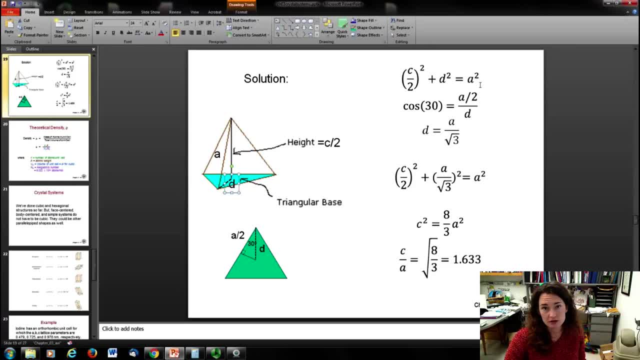 here I have C- over 2 squared, plus D- squared equals a squared. right now I can also look at this triangle right here. okay, this is the base of my pyramid all right now, this would be one of the legs of that triangle and, of course, if I draw, 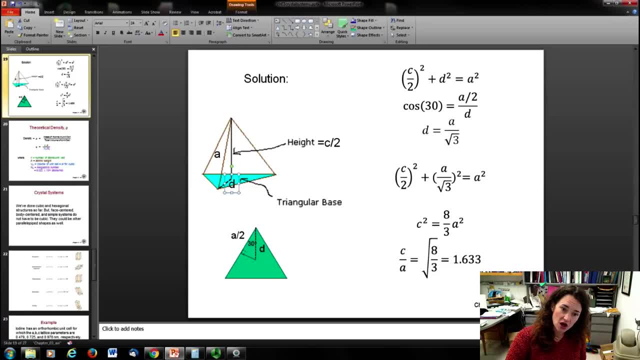 a line halfway along that and then connect it to the midpoint of the triangle. then I can form a little right triangle right here. so each one of the angles in an equilateral triangle is 60 degrees. half of it would be from the plumb line from here to here. so that's half of that is 30 degrees. so I've got a. 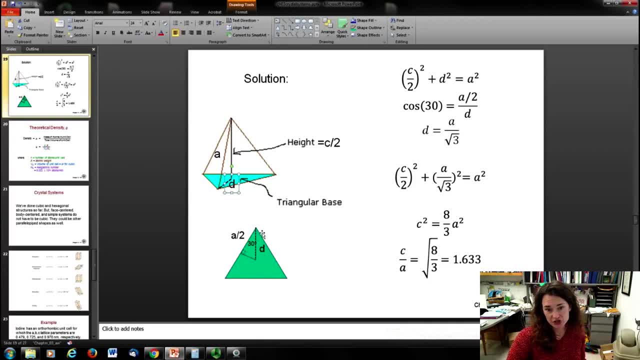 little right triangle right here, with sides A over 2 and then a hypotenuse of D right here. okay, so I can set up a cosine relationship. the cosine of 30 degrees would be A over 2 over D, and then I can solve. solve for what the 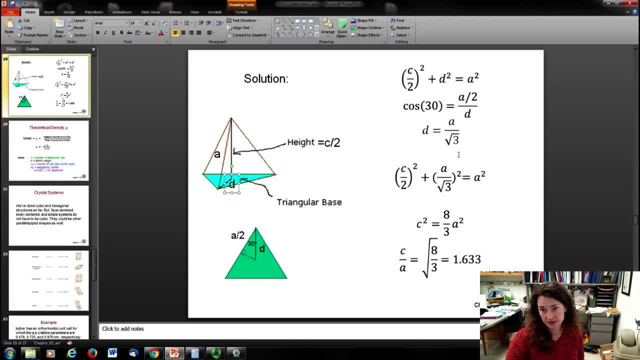 cosine is solve for D and I get D is equal to A over root 3. now from that I can plug it back into my earlier relationship for my Pythagorean theorem. okay, and then I've gotten rid of one of my variables. so I have C over 2 squared plus D squared, which I'm now subbing in A over root 3. 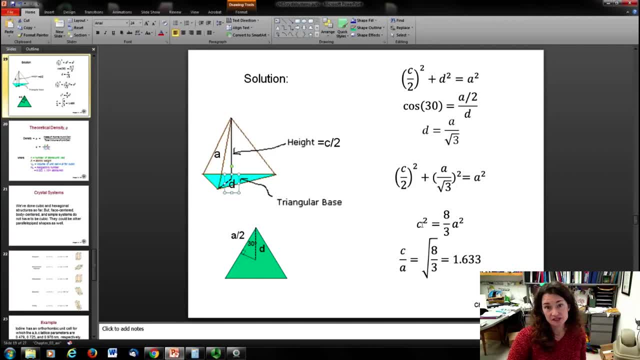 squared is equal to A squared and now I can solve for C in terms of A. so when I do that, I get C squared is 8 thirds A squared, and then solving for C over A, taking the square root of both sides, I get C over A is the root of 8 thirds. 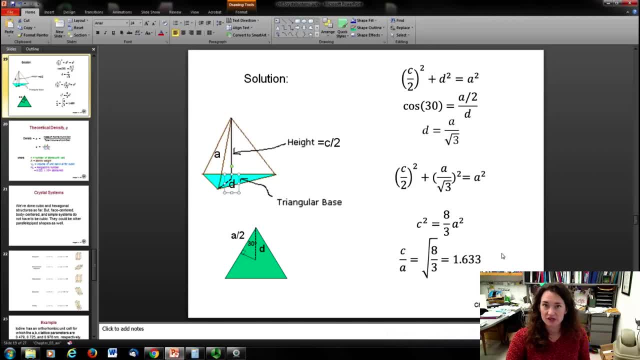 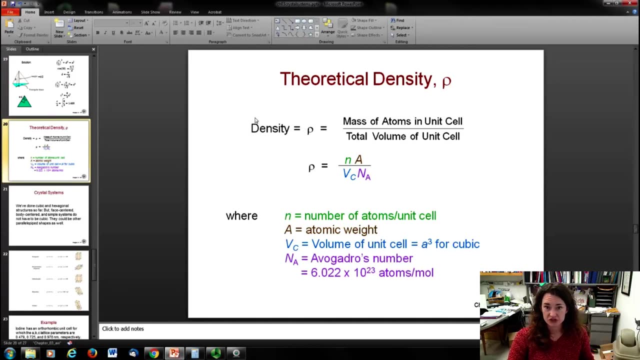 which is 1.633. so that gives us the ratio that it was asked for in the problem. yet again, probably a good idea. pause it, stare at it, make sure you get it. we can also compute the theoretical density for any crystalline structure. now the thing is, it's a theoretical. 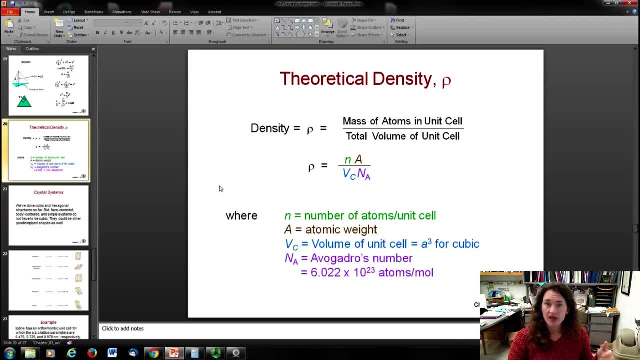 density, because this assumes absolutely no defects and, as we'll see in later chapters, there are lots of defects. so usually your theoretical density will be more dense than your actual density for your material because of the defects in the crystalline solid. so we're gonna use rho as the symbol for our density and 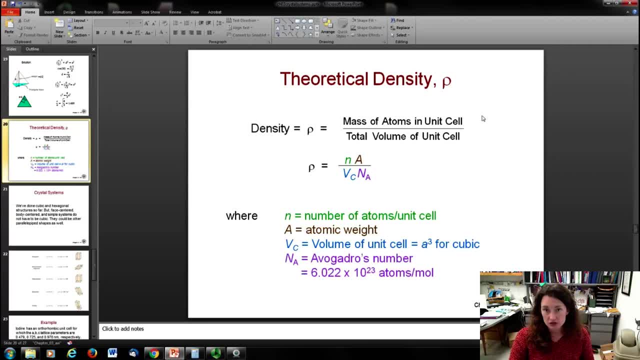 rho will be equal to the mass of the atoms in the unit cell divided by the total volume of the unit cell. okay, so that will give us a unit of kilograms per cubic meter in SI units, or sometimes grams per centimeters cubed. just use because it's convenient now to find this mass of the atoms in the cell. you. 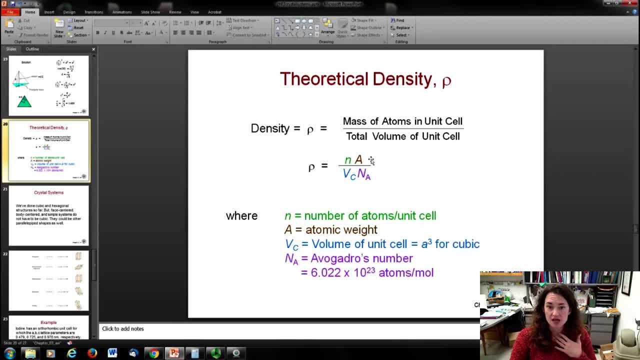 multiply the number of atoms per cell times, the atomic weight of each atom, and then you multiply that vários por semana de los átomos por el�el shift cross곳. Then you divide by the volume of the cell, a cubed for a cubic cell, and then you multiply. 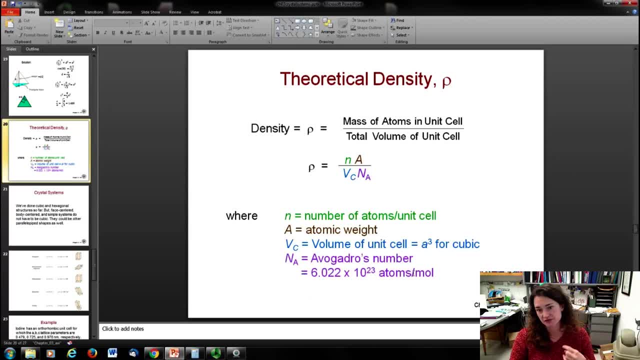 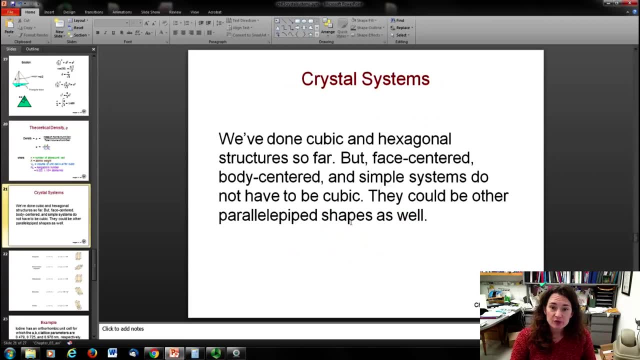 that times Avogadro's number, 6.022 times 10, to the 23rd atoms per mole. Okay, now we've done cubic and hexagonal structures so far, but face-centered, body-centered, cubic, simple systems don't have to be cubic, okay. 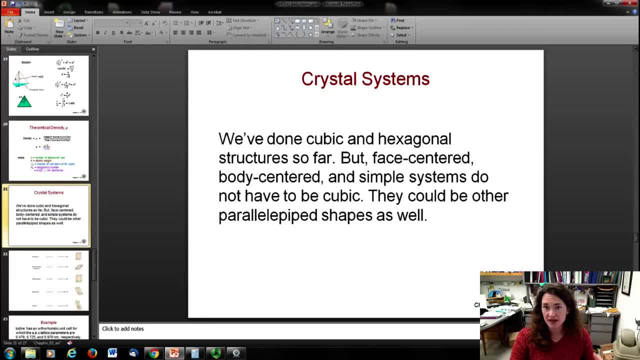 They could be other parallel pipette shapes as well, And this often happens, especially if you have, instead of just a single type of atom in your crystalline structure, you have some blend or alloy. then you're going to get more complex-looking structures. 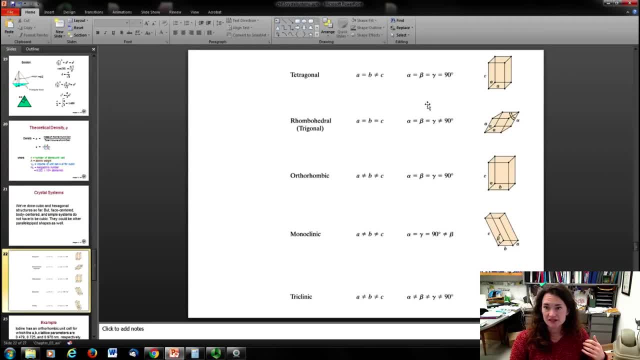 So here's some of the possibilities. This is a tetragonal structure right here and in the tetragonal structure you have a square on the bottom, but then the height of your upright solid isn't the same as the length of the base. 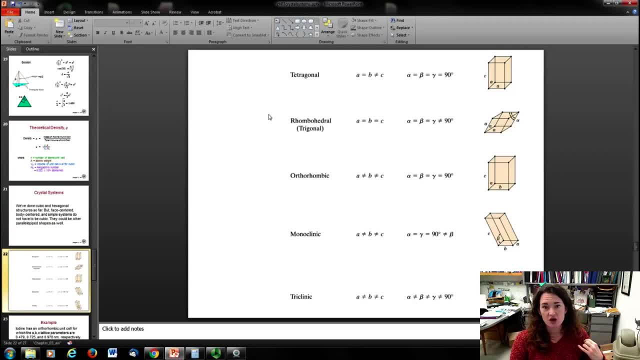 All angles here are the same. Here are 90 degrees. You could also have a rhombohedral structure or a trigonal structure. They are all. the lengths are the same, but the angles don't have to be 90 degrees. for 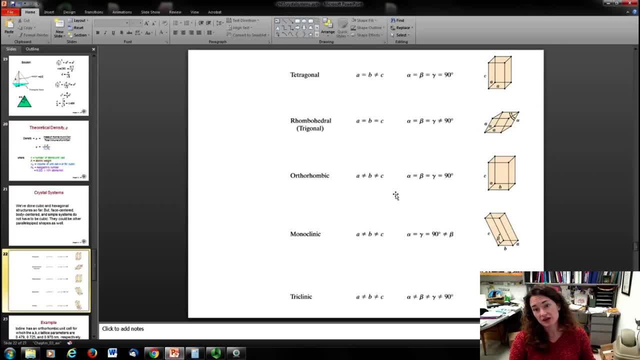 all of them. You have an orthorhombic structure where none of the lengths of the sides are the same- A, B, C, all different, but they are 90 degrees. You can have a monoclinic structure where A doesn't equal B, doesn't equal C, but not. 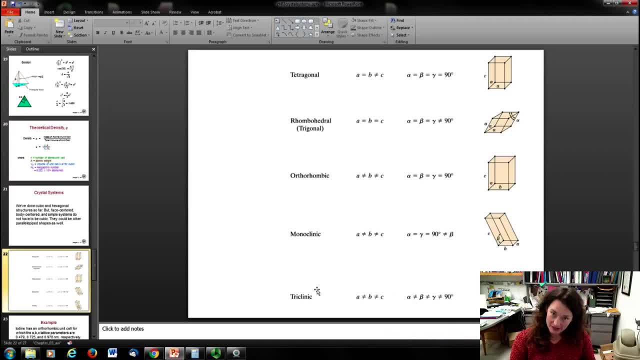 all the angles have to be 90 degrees, Or you can have a triclinic structure, You can have a monoclinic structure where A doesn't equal B doesn't equal C and none of the angles are 90 degrees. 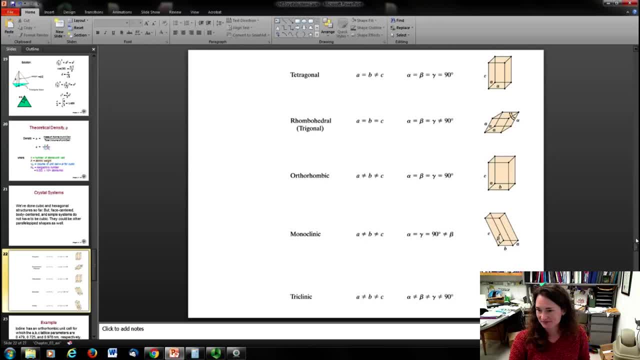 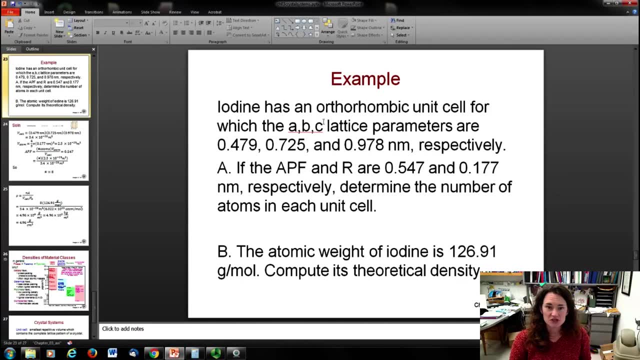 So you can have all these different choices of structure. All right, so let's do an example. problem: Iodine has an orthorhombic unit cell for which the ABC lattice parameters are 0.479, 0.725,. 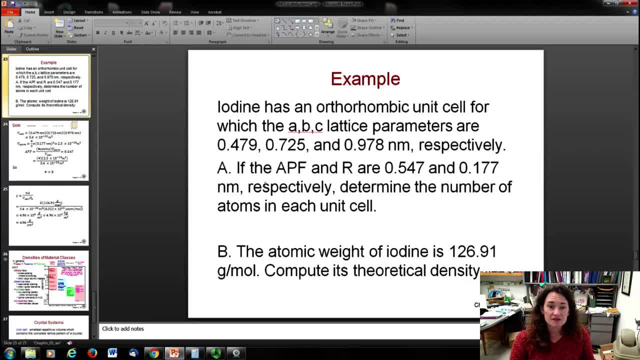 and 0.978 nanometers respectively. If the atomic packing factor and the radius are 0.547 and 0.107 nanometers, then you have an orthorhombic unit cell for which the ABC lattice parameters are 0.479,, 0.725, and 0.978. 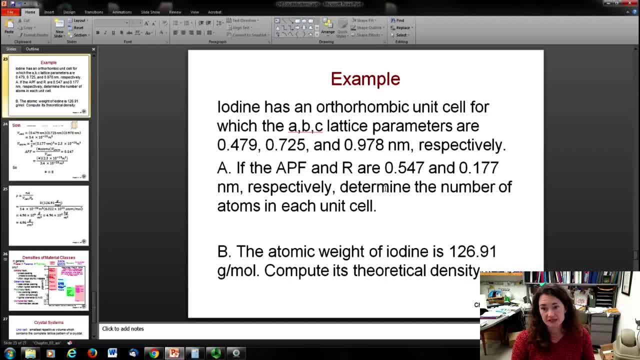 nanometers respectively. If the atomic packing factor and the radius are 0.177 nanometers respectively, then determine the number of atoms in each cell. And the atomic weight of iodine is given as 126.91 grams per mole. so compute its theoretical. 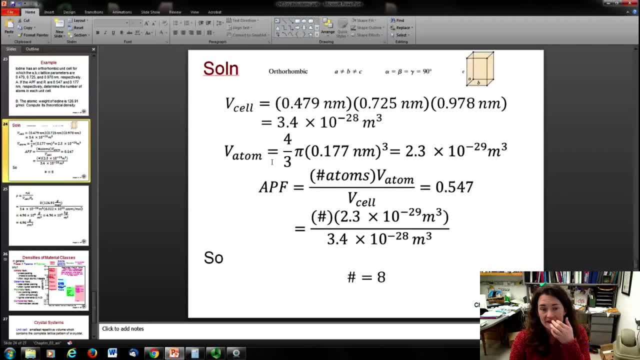 density. OK, so first of all let's compute the volume of the cell. This is an orthorhombic. It looks like this sort of upright solid here: A, B and C are not the same, but they're all 90 degree angles. 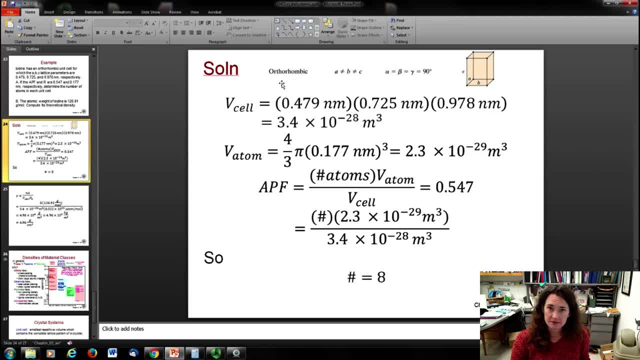 So here you just multiply length times, width times, density, So you have 0.479 times 0.725 times 0.978 nanometers for each one of those things. If you write it out so that 0.479 times 10 to the minus 9, then you can get it in terms: 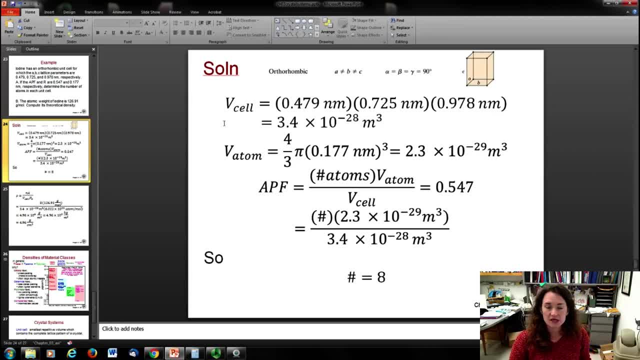 of meters cubed, if you want to, And then you can multiply all three of those things. Then the volume of the cell is 3.4 times 10, to the minus 28 cubic meters, The volume of a single atom. it gave you the radius of the atom as 0.177, so we're going. 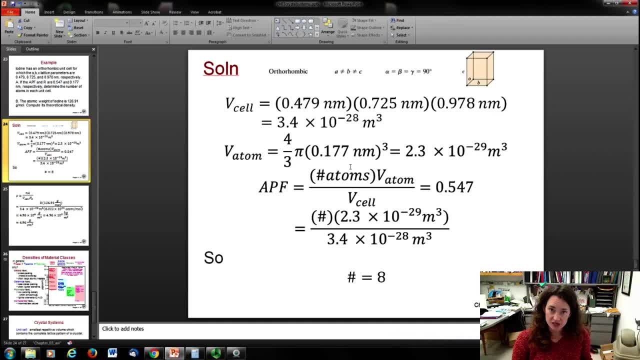 to use 4 thirds pi r cubed as the volume of a sphere, For the volume of our atom as an approximation to that, And when we do that we get 2.3 times 10 to the minus 29 cubic meters. 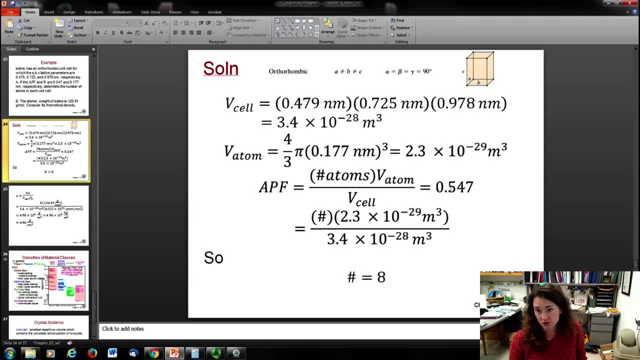 So that means that we know our atomic packing factor. It's 0.547.. And we can use the formula for the atomic packing factor to calculate the number of atoms Because, remember, the APF is equal to the number of atoms times the volume of an atom. 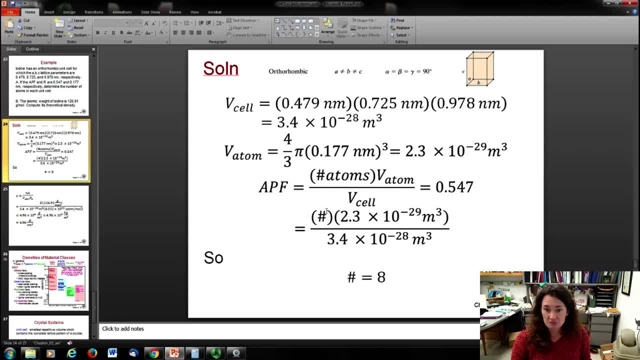 divided by the volume of the cell. So here we have the number times 2.3 times 10 to the minus 29.. Divided by 3.4 times 10 to the minus 28.. We set that equal to 0.547.. 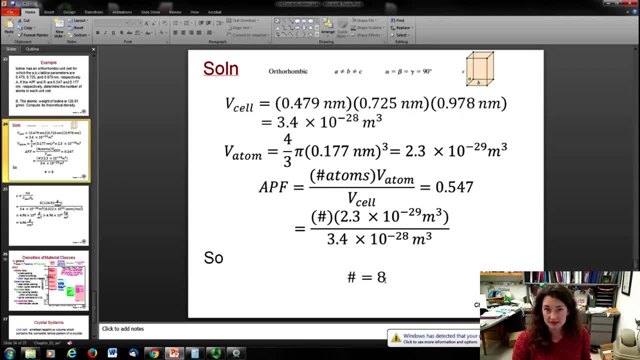 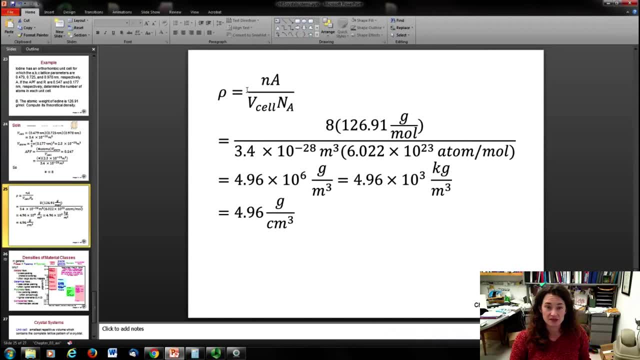 We solve for a number, And that gives a number approximately equal to 8.. Now we can also use our formula for our theoretical density and solve for it. So now we know the number of atoms in the unit cell. It's 8.. 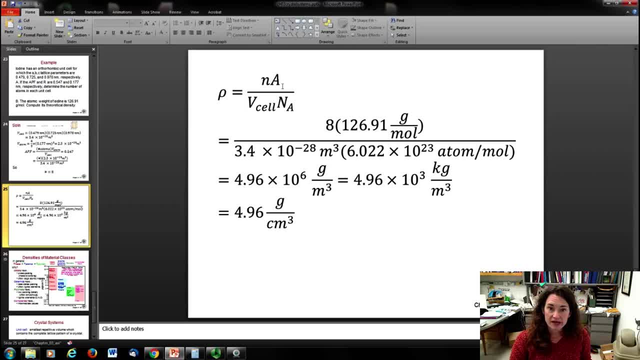 We solve for that in part a, So we can plug that in. Here is the atomic weight. It's given in grams per mole. So we're going to multiply times that And then we divide by the volume of the cell, which we already solved for, 3.4 times 10. 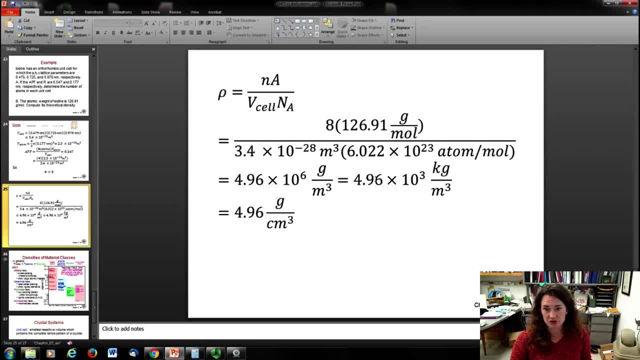 to the minus 28.. And then we multiply by Avogadro's number. You can see here the purpose of Avogadro's number is as a conversion factor, Because if you have your atomic weight in grams per mole, then you need to convert that. 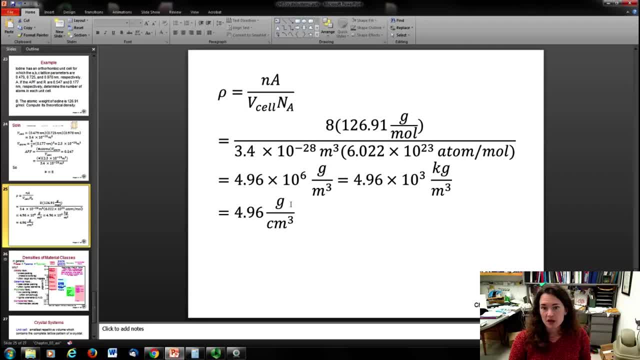 out Okay, So that's what we've done here. Multiplying through during your dimensional analysis, you can see that you get 4.96 times 10 to the 6 grams per meter cubed. That's not typical For how you give a density. usually you give it in either kilograms per meter cubed. 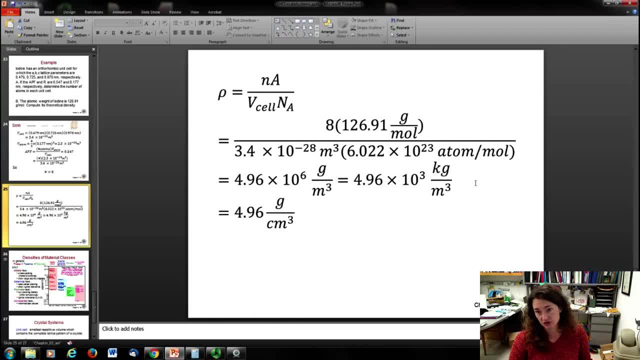 To convert that, you just divide by 1,000, and you've got it in terms of kilograms per cubic meter, 4.96 times 10 to the 3 kilograms per cubic meter. Another typical unit for density is grams per centimeters cubed. 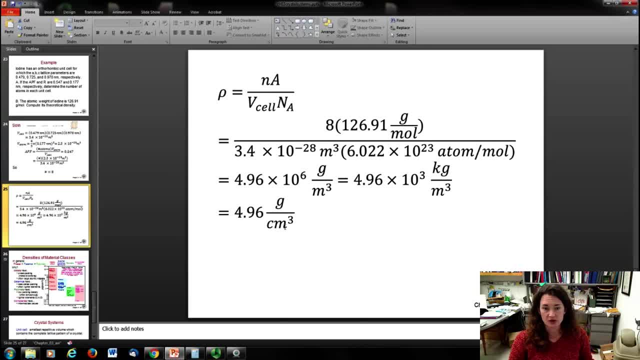 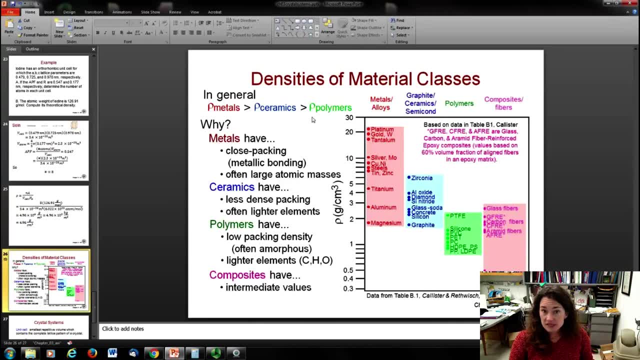 So I've done that conversion here and you get 4.96 grams per cubic centimeter. All right, So that's our theoretical density. Speaking of density, Speaking of density in general, metals are more dense than ceramics, which are more dense. 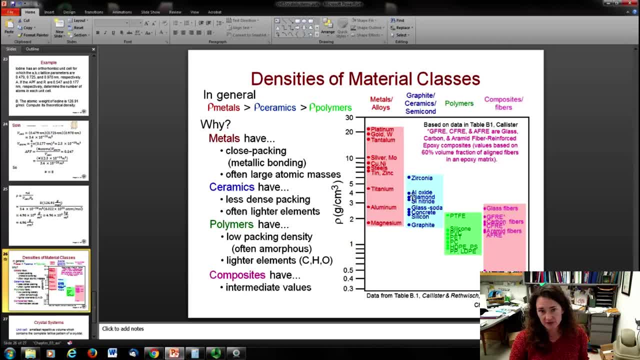 than polymers. in general, There is some overlap, Why? Well, metals have close packing, they have metallic bonding and they have very large atomic masses, Right? So if you have a large mass divided by the same volume, you're going to have a higher. 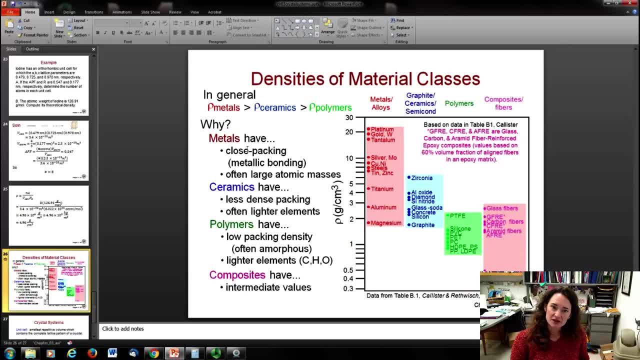 density. Also, metals undergo that metallic bonding where they have the ionic cores surrounded by the electron C Right, So that causes the bonds to be a little shorter. Ceramics, however, are bonded, usually in ionic-type bonds, and so their bonds are going to be. 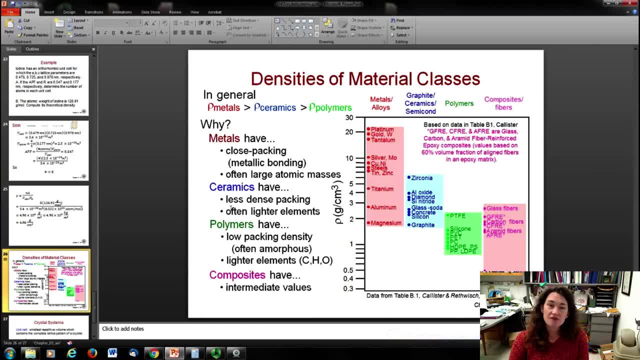 a little larger than the electron C, And they're often made of lighter elements, of course. So that means that the mass that you've got on the top of the numerator is a smaller number, so you have a lower density. Polymers have the lowest packing density. 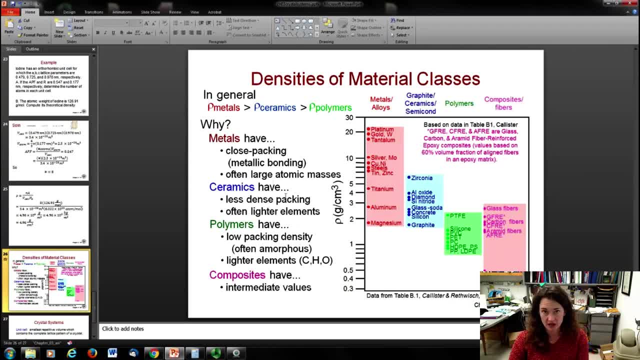 They generally are composed of carbon, which is a very light element, or they have a lot of carbon in them, So that contributes to a low density. But also they're often amorphous, which means they're not going to be as tightly packed. 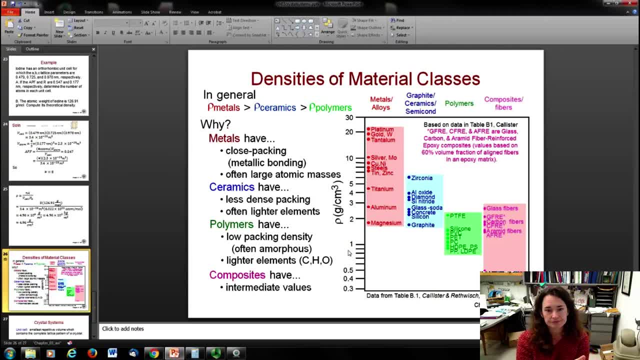 and those inter-atomic bonds are going to be a little larger, And then composites, of course, are a blend of all the materials, And so they're going to have intermediate values for all of these things, because they're going to be, say, for example, a blend of a metal and a polymer or something like that.